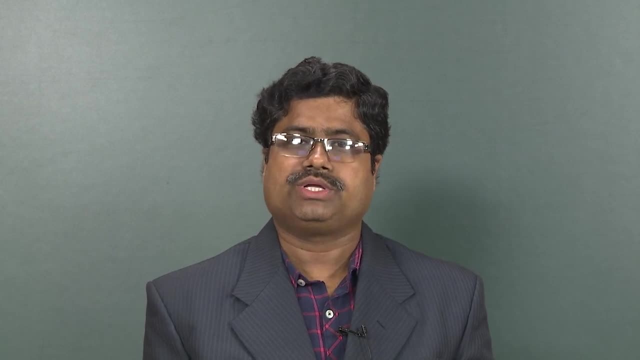 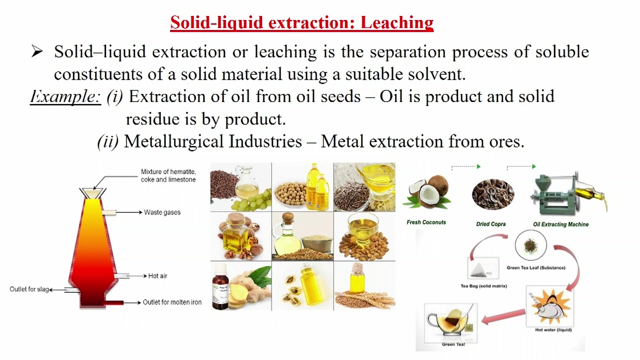 to the solubility difference of the solute in different phases, that is, in the carrier solvent and the extracting solvent. the solute was transferred from this carrier phase to the extracting phase. In this solid-liquid extraction, we will be discussing the almost similar procedure, except that the in place of this carrier solvent. 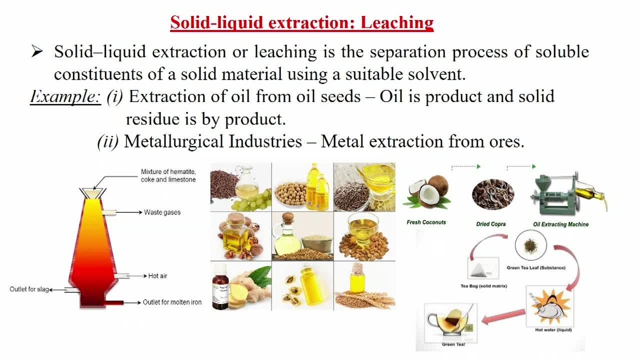 in case of the solid-liquid extraction, there will be one. we can this solid material, or we can say this one, that inert material, or we can say this one, the residual which will be left out after the extraction process. So we can say this one, leaching, that is one. 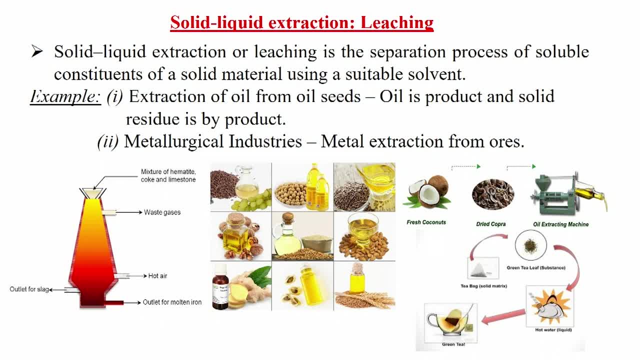 solid-liquid extraction process, that is, the separation phase. So this is the material process of soluble constituents of a solid material using a suitable solvent. So inside a solid material, suppose one particular target component is there which can be solubilized in the particular suitable solvent. so there are so many examples we will be discussing. 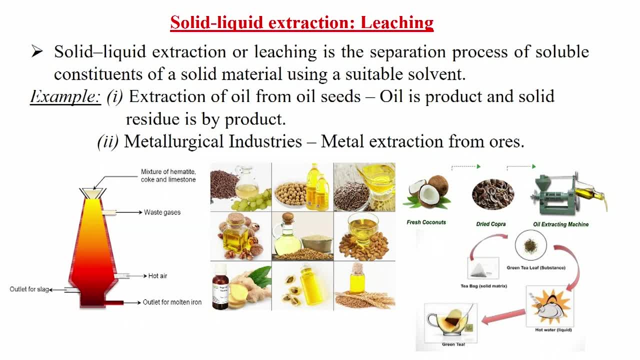 few examples of the liquid, solid-liquid extraction process like this. we can say this one. the one common example is the extraction of oil from oil seeds. suppose this oil contents mostly say 15 to 20 percent oil and the rest amount is this inert, or we say this one, the residue. 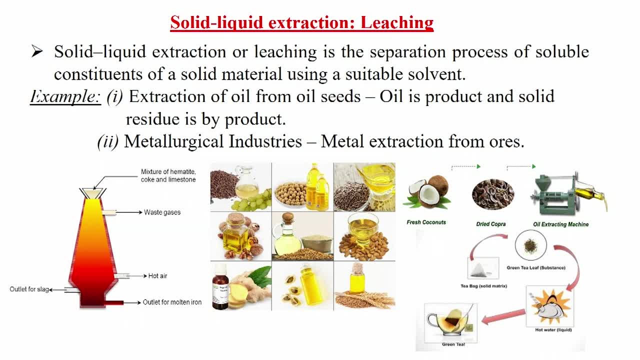 so this, that oil content can be extracted using this particular organic solvent. where this oil is solubilized And in metallurgical industry say, metal extraction is done From the ores. so here there are some examples like this. we can say: suppose in the metallurgical 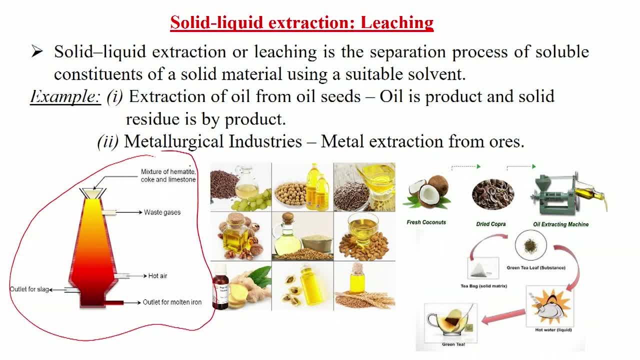 industry say, suppose the different mixture of hematite, or we can say this one, the source of this metal is added and coke and some limestone, these are added. so inside this one we can say this: inside this blast furnace. so the ores are extracted with the help of this coke. 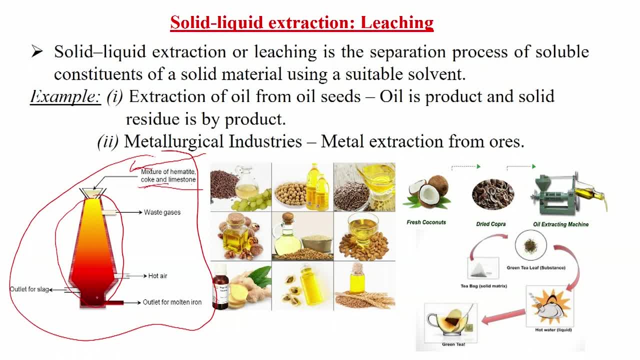 and say limestone, And then we can say this one from the outlet, this molten iron that is separated as the product, and we can say this slag, which is- we can say this one- left out, that is, we can say this one as under flow. So we will be discussing about this whenever we will be discussing about the solid-liquid. 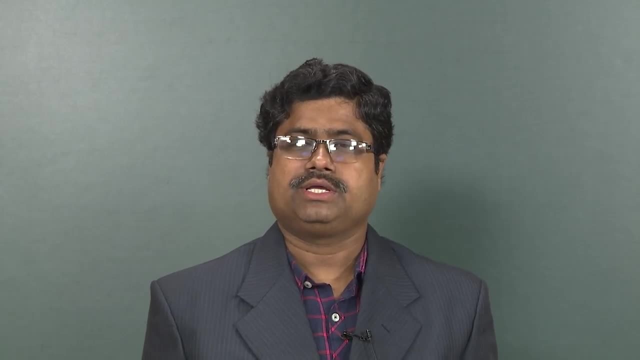 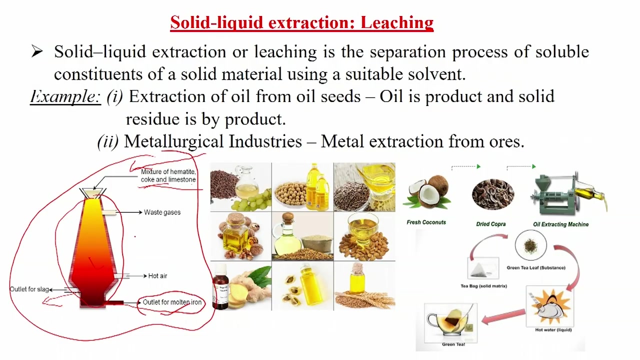 extraction. so two phases are added in, say we can say this one in any extraction unit. or we can say this leaching unit like say this is one leaching unit, So two phases, like this hematite coke and limestone, these are added and say this one. 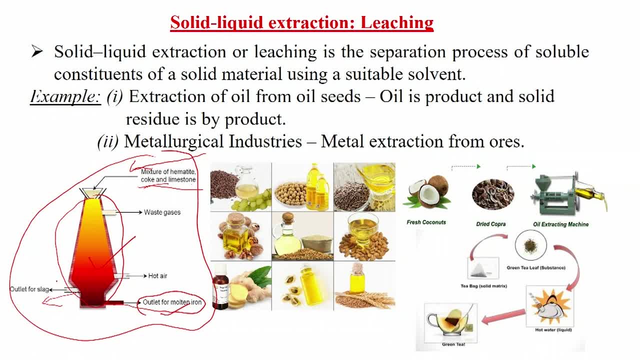 it is separated into two different phases like this. one will be this overflow, this is, say, outlet for slag, that is the underflow. and whatever this outlet for molten iron, that is called, say, overflow. And if we say this essential oil, and we can say this volatile oil, separation from this. 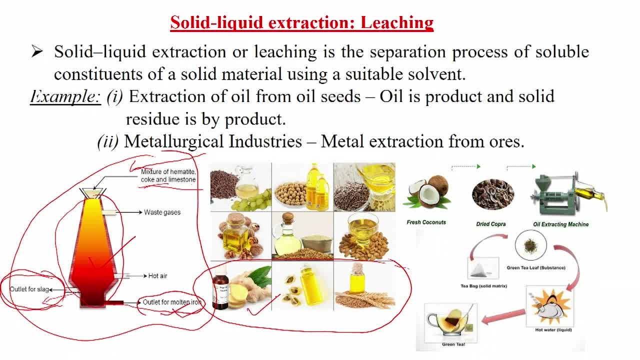 say, ginger, like this, in terms of, say, 6 ginger oil. that is done frequently using this supercritical fluid extraction. So there, actually, we get this 6 ginger oil. or we can say this, some essential oils- There are so many this one oils- these are recovered using this, say, solid liquid extraction. 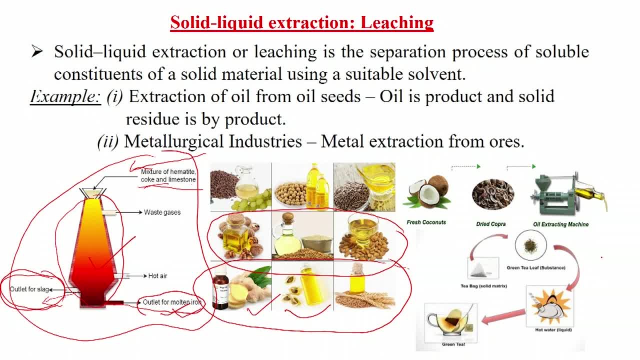 processes, Like also say this one in our daily life, say we generally take this tea, like this tea bag, or we can have this solid matter Matrix is there, or we can say this: only tea is there and we are adding this one in this. we can say this one inside this hot water. 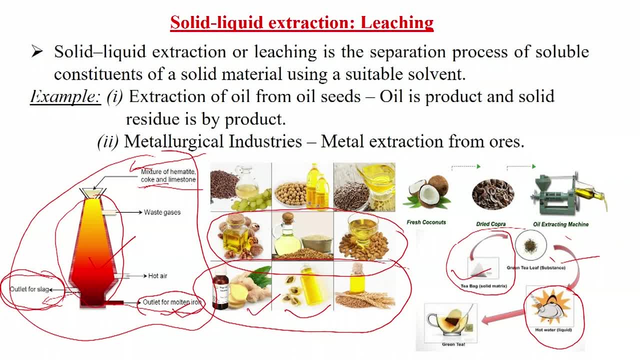 Then this: from this solid tea, this, we can say this one: whatever this caffeine that is separated. that is another example of this leaching process. Then we get this green tea. So this is, we can say this one, that is coming out and whatever is left of, we say this one: 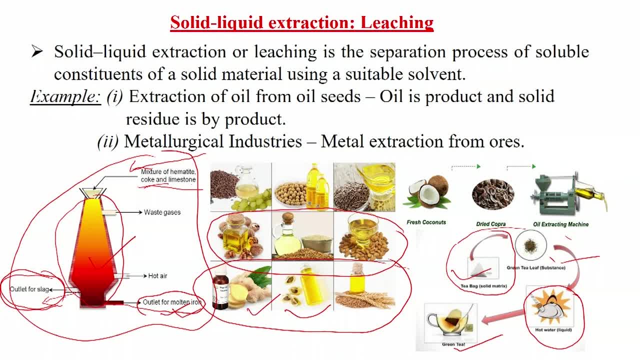 the whatever the residue is obtained after this leaching process. we say this one as the residue. So there are so many like this, say, from fresh coconut. also, we can get this coconut oil using the similar type of, we can say, separation process. this is, we can say, leaching. 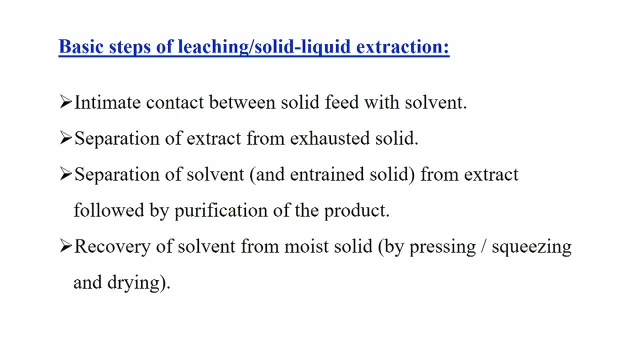 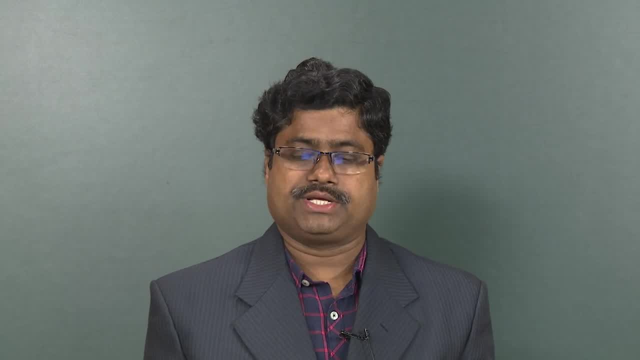 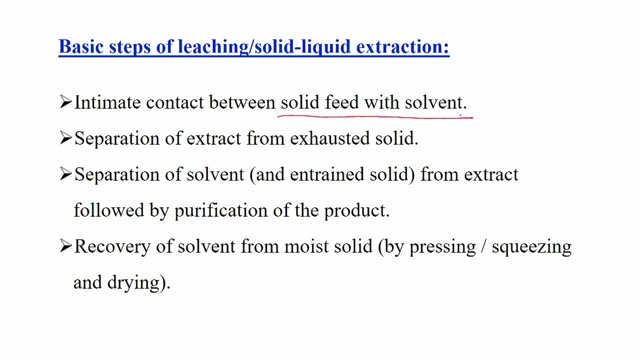 So the basic steps of the leaching or, we can, solid liquid extraction. this is almost similar to that of the liquid-liquid extraction process, with some amount of modification, So alterations like this. first step is this: intimate contact between the solid feed with the solvent. 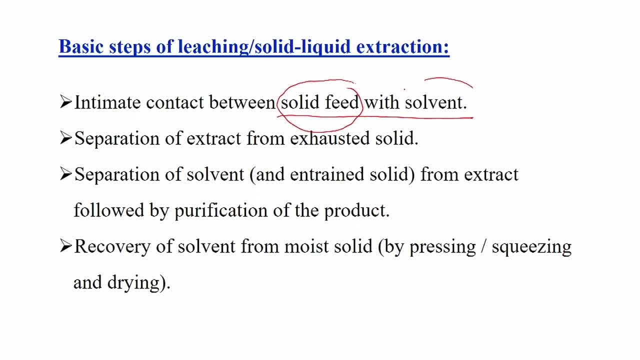 So here we have this, solid is there and we are adding this liquid. So solid is contacted with the liquid. So that is why it is solid-liquid extraction and inside this solid, say, one target component is there which can be solubilized inside this solvent. 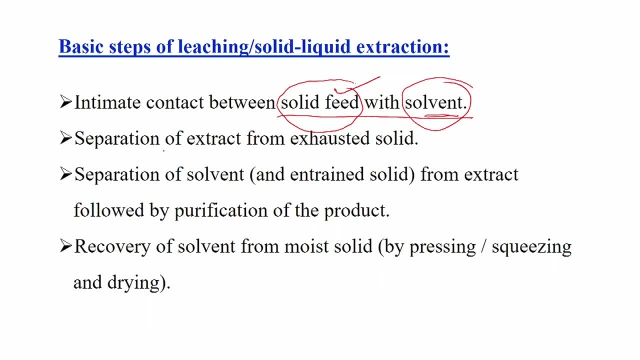 Then separation of the extract from the exhausted solid. So now then we need to say, Suppose this is our leaching system, suppose we have this feed, and to say we have added their solvent, then we are allowing the system to be separated into two. this parts one: we 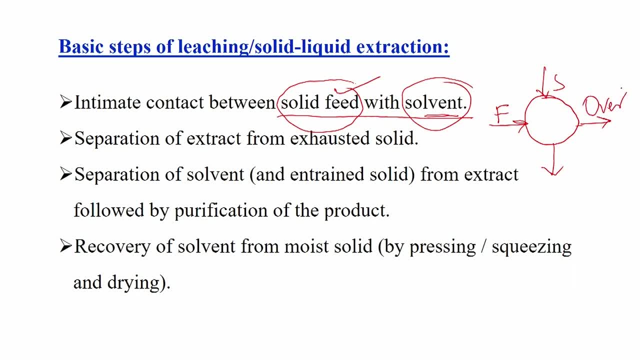 can say this: one overflow, then another one is called underflow. So we need to separate the extract. this overflow is nothing but this extract. And we can say this one: whatever exhausted one is called this underflow, The separation of the solvent. we can say this one and some entrained solid may be there. 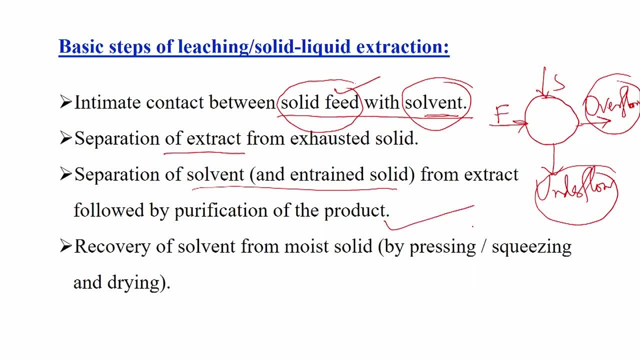 from the extract, followed by purification of the product, like extraction process. the similar way, recovery of the solvent from the moist solid, just from here we can say this one, by pressing, squeezing and drying. So this one, we can recover solvent from both this overflow and underflow, just like extraction. 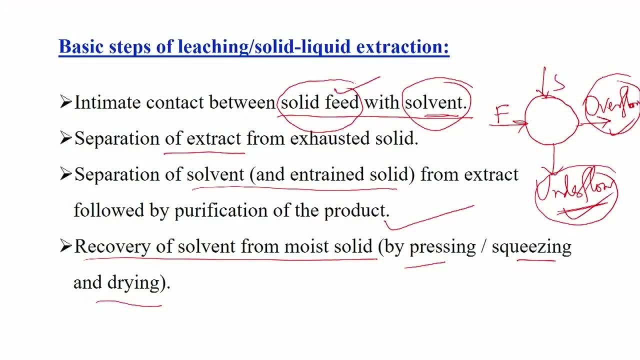 process. So from this extract, this is equivalent to overflow, is equivalent to extract and underflow is equivalent to raffinate, So liquid-liquid extraction also. we followed the similar steps. they are the last two steps where, like this, recovery of the solvents from both the extract and raffinate phases. 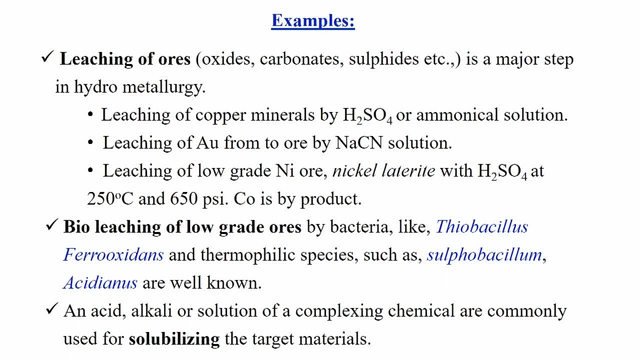 Again, we are this one discussing the few examples, actually not in detail, but we will be discussing the overall: the single stage process and the multiple stage process. So this is the first step, So this is the second step, So this is the second step and this is the third step. 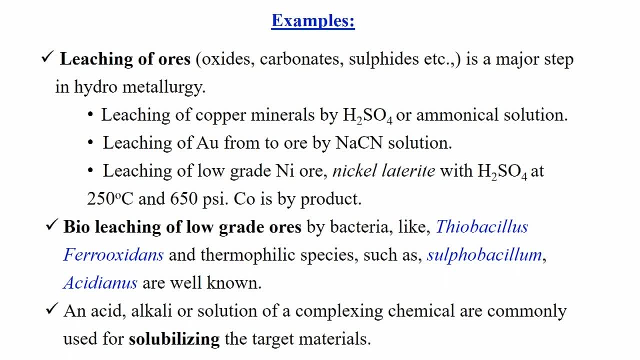 So we will be discussing the two stages in the this one next few slides. So suppose the leaching of this ore, that is we can say this oxide carbonate, sulphite et cetera- is a major step in hydro metallurgy. They are leaching of this like copper minerals by sulphuric acid or ammoniac solution, or we. 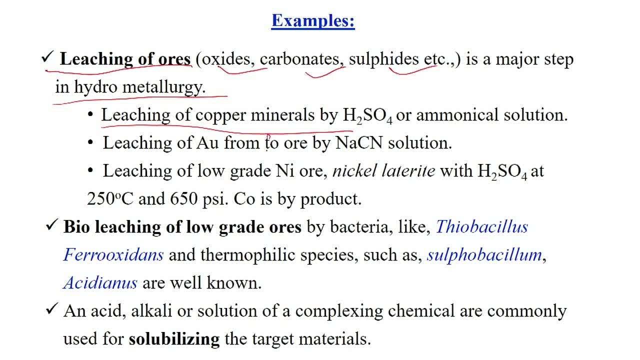 can say the leaching of gold from the ore by sodium cyanide solution. and then we can say this one leaching of low grade nickel ore- like we can say, it is called as nickel laterite- with sulphuric acid at 250 degree Celsius and 650 psi, and there actually cobalt is the byproduct. 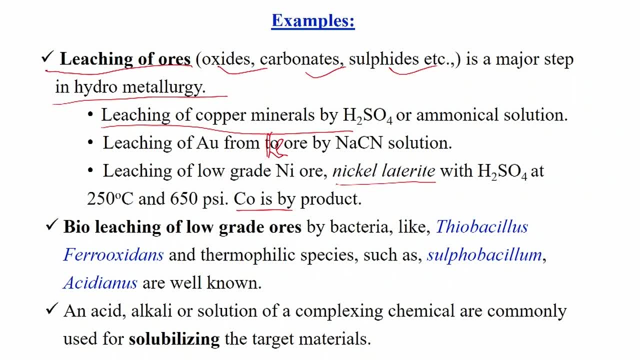 So in case of this leaching, we will be getting sometimes this useful byproducts, like whenever we have leaching of oil from oil sheets, whatever inert actually we will be getting, or we say cake, that is will be the byproduct that will be used as the fertilizer, or we can say for. 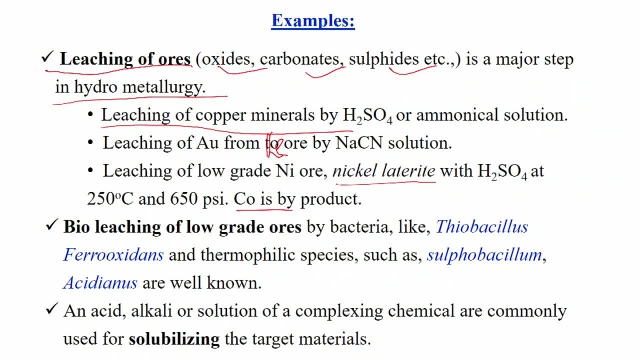 the- we can say this- cattle, also cattle field. these are actually used as the fodder for those, we can say like cows or buffaloes. And another example, like this bio leaching of this low grade ores by bacteria, that is, we can say this one: these are the newest leaching applications, that is like thiobacillus phytophthora. 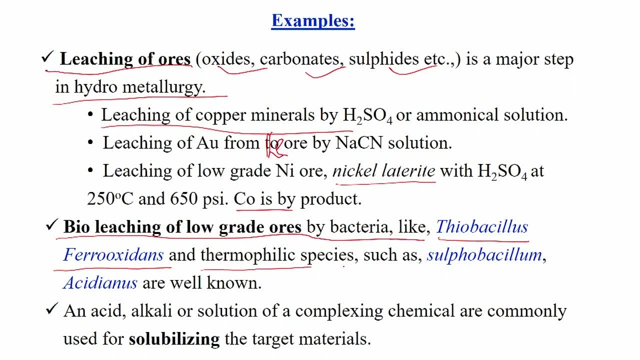 ferroxidans and we can say this one: thermophilic species such as we can say this sulphobasillium or acidinium, are well known there. actually, these bacterias, we can say this one, dissolve the ores, or metal oxides, or say we can say this one from the ores, without the application. 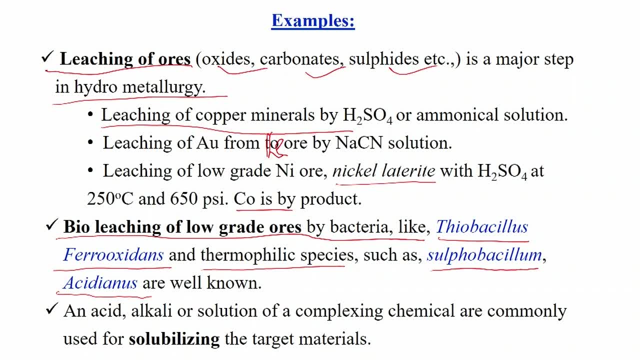 of the chemicals. So this is, we can say, this is the new application of the leaching process, and any acid, alkali or solution of complex in chemicals are commonly used for the solubilizing of the target material. so in that case we can say this: one extraction of this target. 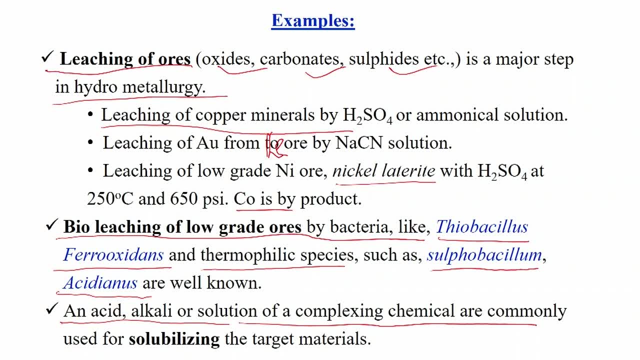 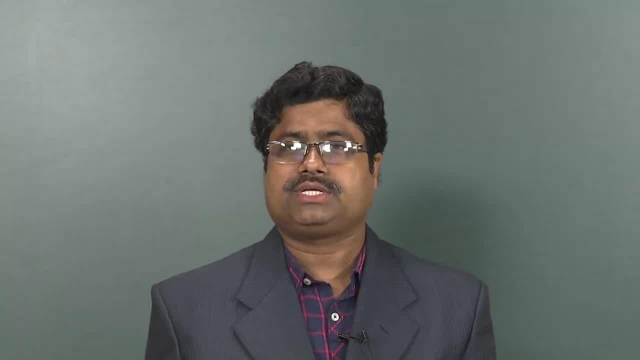 component becomes very high. And another example that we will be discussing in detail: like this: supercritical fluid extraction. there the target component is efficiently separated using the supercritical fluid. like this- we can say supercritical carbon dioxide in general- to get the we can say this one: 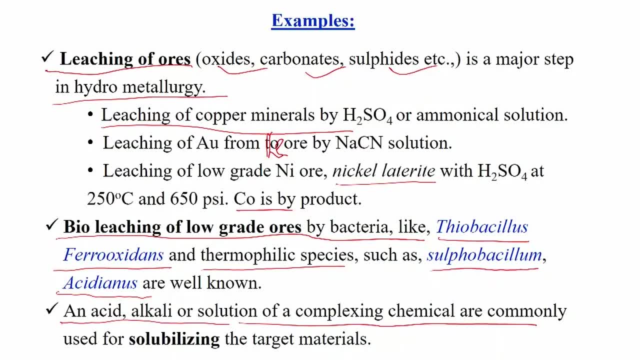 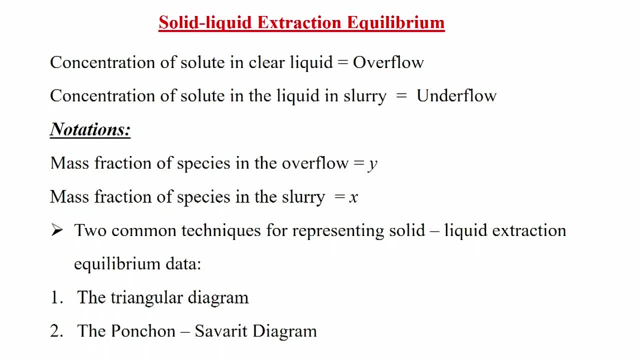 maximum extraction output. this one out of the process. Now we will be discussing the solid-liquid extraction equilibria, that is, the similar to that of the liquid-liquid equilibria, like this. here we will be discussing about the concentration of the solute in the clear liquid. we can say this: one overflow, that is equivalent. 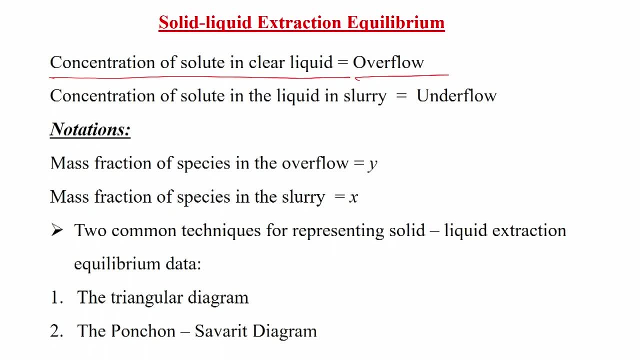 to. we can say this one: extract in the liquid-liquid extraction Extraction process and then concentration of the solute in the liquid, this one in slurry. or we can say this one in inert material or in the cake that is termed as underflow. 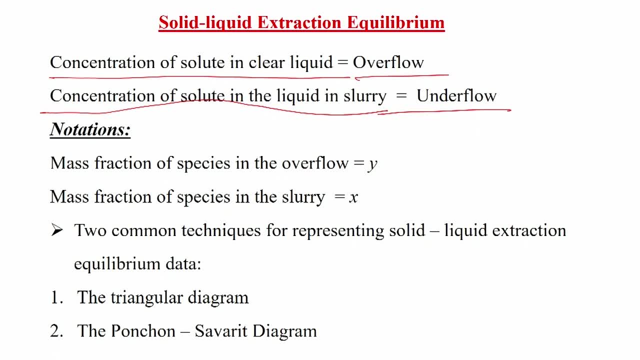 So when we say that the system, this solid-liquid extraction system, has reached its equilibrium, means the we can say this one concentration of the solute in the overflow and concentration of the solute in the underflow. that will become same and we will be using some notations. 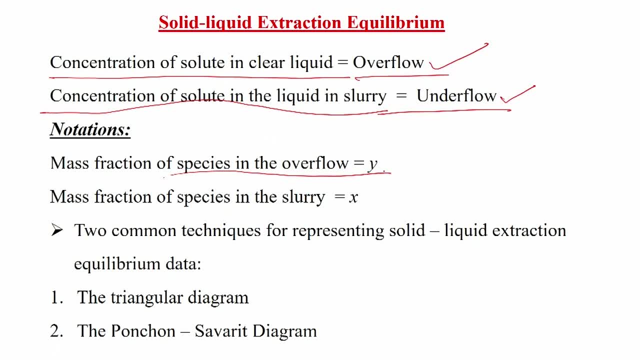 like this. mass fraction of the species in the overflow will be like Y say. here also we have ABC concept- we will be discussing just now, we will be discussing this one- and mass fraction of the species in the slurry, that is, will be denoted as X. 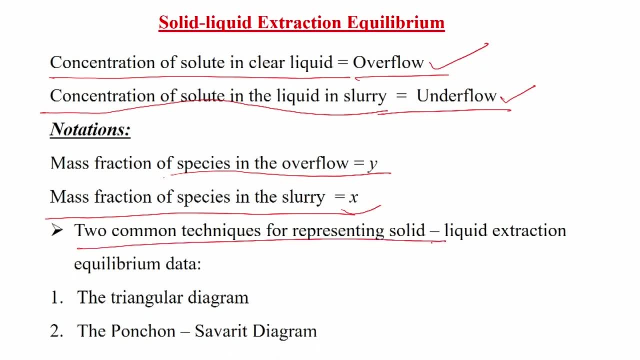 So two common techniques actually for separating solid-liquid extraction equilibria data Are like triangular diagram. in most of the cases, we will be using this right triangular diagram we will be using, and another is this Ponchon-Savarit, that is, we can say this one. 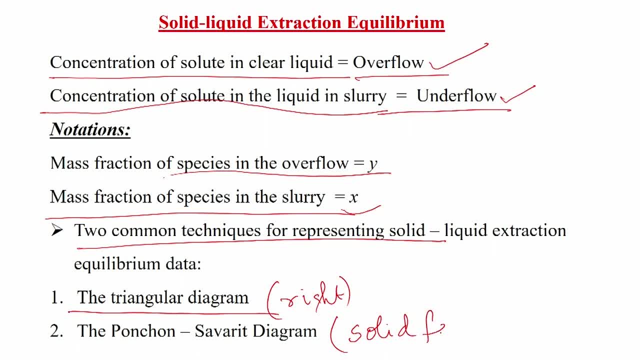 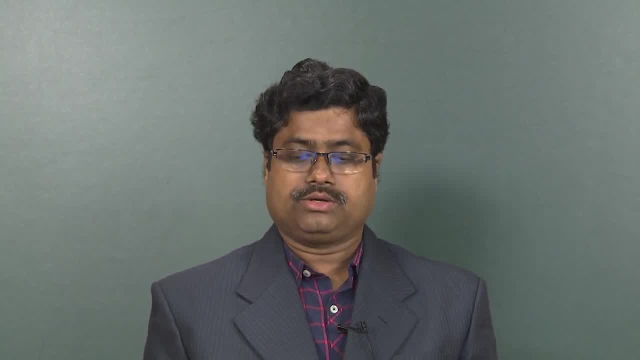 solid free basis. It is equivalent to. we can say this one, just like in case of this liquid-liquid equilibrium, that is, we can say this one: solvent free basis. So you see, these are all almost equivalent. actually, we will be discussing whenever we will be solving the problem. 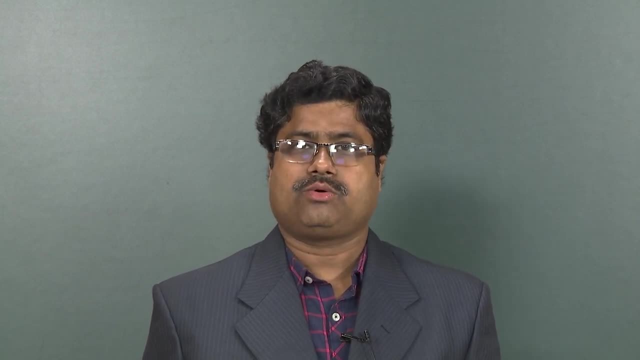 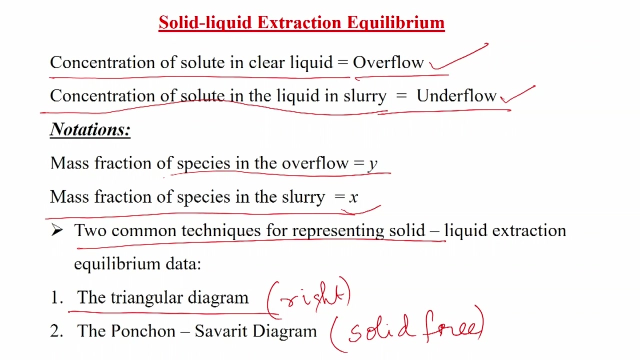 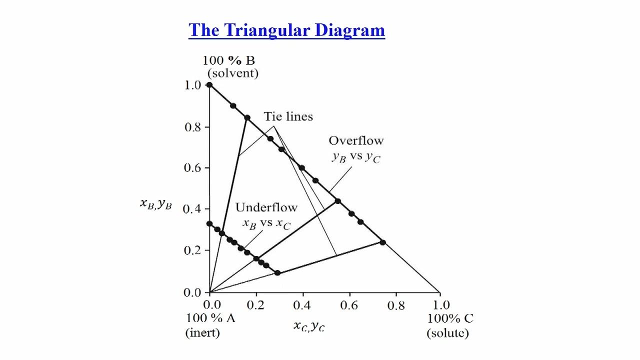 We will find that the these two processes are almost, so we can liquid-liquid separation process, or liquid-liquid extraction and solid-liquid extraction process. wise, these two processes are, or we can say the unit operations are- almost similar. So the first, we can say this: one set of this, we can say diagram, that is, we can say this: 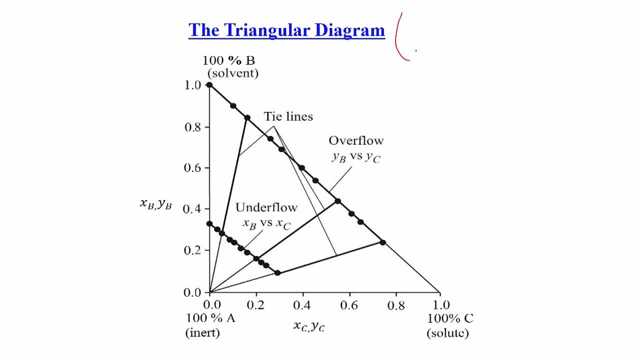 one triangular diagram, That is, we can say this: one right triangular diagram, we can say this: one equilateral, also triangular diagram also we can use Here. you see this: the target solute is placed in X axis and we can say this one solvent is placed in the Y axis and we can say this one. just, it is also we can say to some extent: 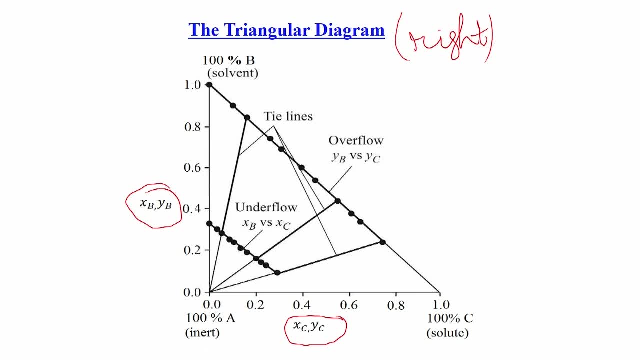 inverted one compared to the liquid-liquid extraction. One can use also C at the tip, also means the apex here, And we can, one can keep B also here, Then otherwise this, we can say: this one concept wise, this is also same. So whatever the equilibrium data points are there with this underflow and overflow, these 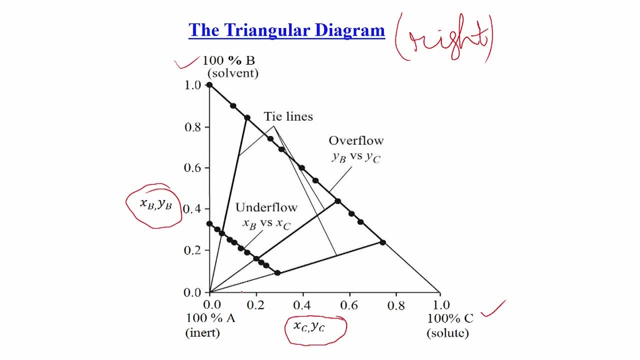 are all interrelated with this straight line. One important point is there: in case of this leaching process, all the tie lines will move through this 0: 0. So that it has one additional advantage. Thank you, Like whenever we will be drawing any straight line, starting from this 0: 0 point means say: 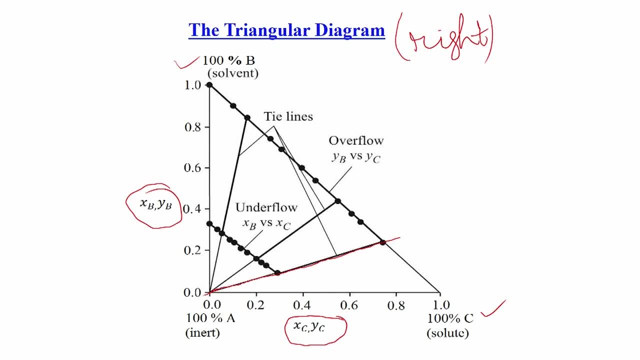 whenever 100 percent inert is there. through this, whenever we will be drawing any straight line, it will cut both this underflow and overflow and these are all tie lines. So that is we can say this one, all the tie lines, whenever we will be drawing any point. 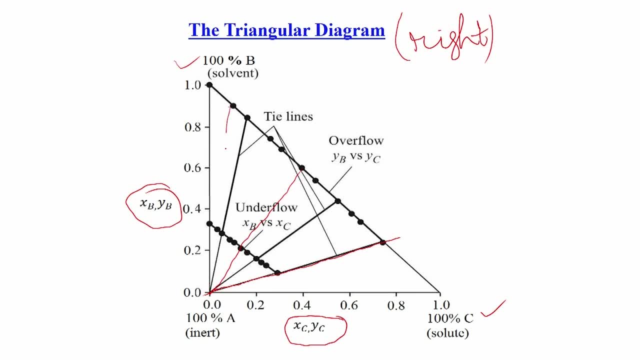 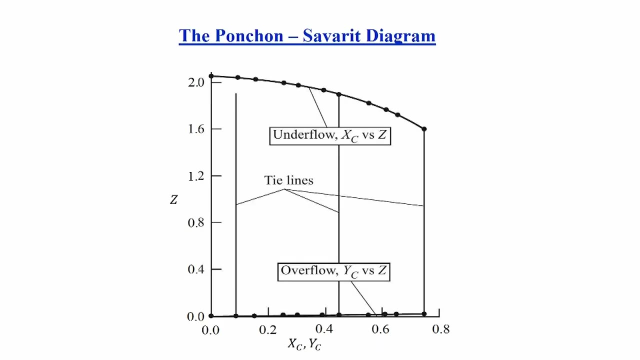 like this and if we extend to 0, so these all are. we can say this tie line, So we can say this B axis as well as this C axis, These are all. also, you can say this one tie line values are there And say another one is called this: Ponchon Shabari diagram. 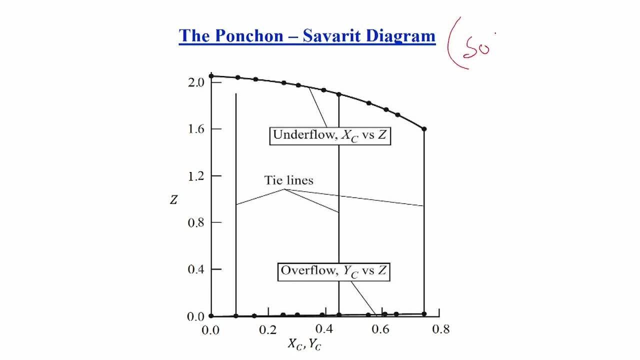 That what we can say, this one, this is solid, free basis. We will be deriving this one how this Z is similar to that of the extraction process also, and XC and YC. This is also similar to that of the leaching process. Here also, you see how it isining up to 0.. 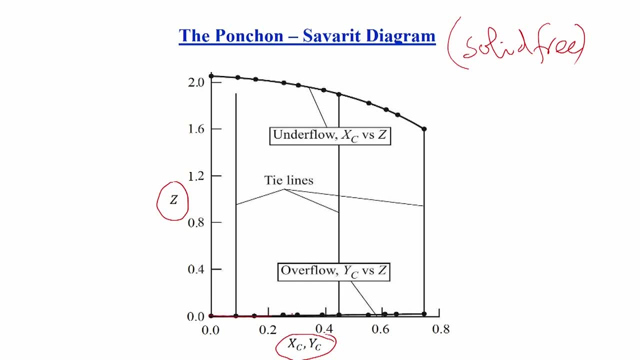 For that we can Galilean drive. Also we can write thisology like it can have similar base relation. see, this underflow will be lying almost in the this one, what is called the C line, and this the underflow will be like this: it will be following this one, but with the value higher. 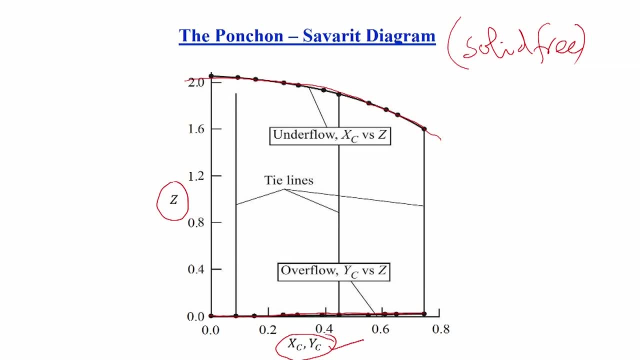 than that 1, because you see we will be, whenever we will be discussing about Z in a solid, free basis. in all the cases for this underflow we will be getting. this Z is always greater than 1. we will be getting- we will be just showing this- what is the Z value for underflow. 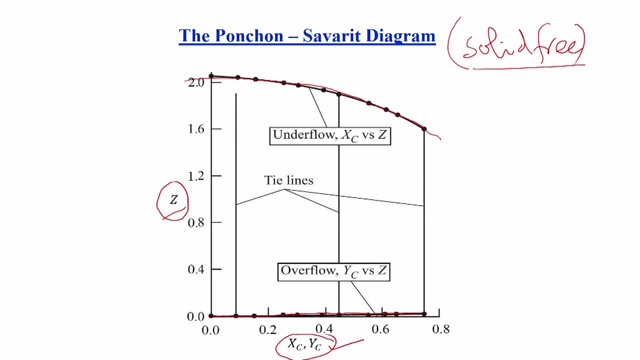 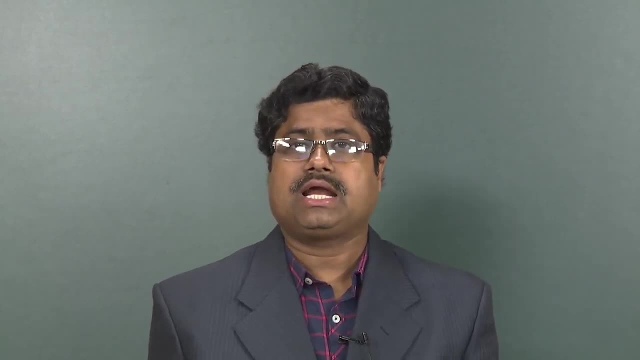 and overflow. and what is the XC capital XC and capital YC? for this we can say the underflow and overflow and say we can say this one whenever we will be using this ponchon-savary diagram. so as it is solid, free basis, so the inert has no effect. or we can say whatever cake. 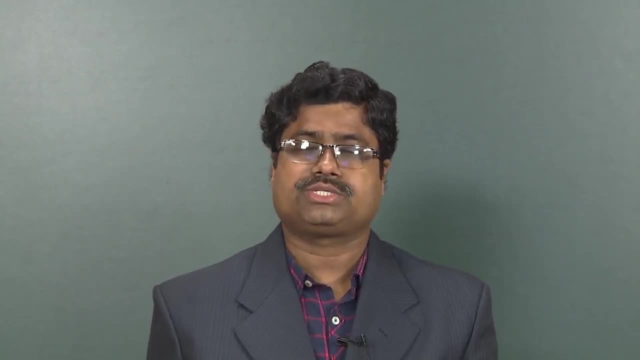 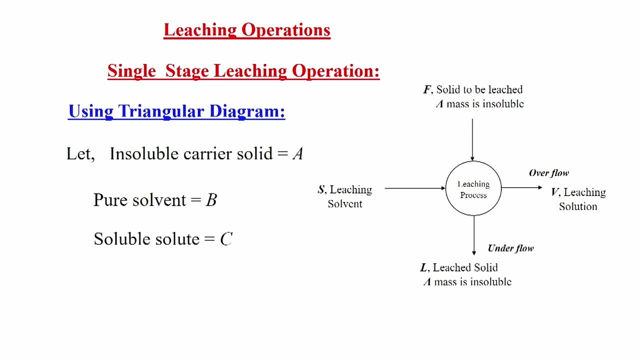 is has no effect on the. we can say this: one calculation Of the leaching process and they say this: one first operation, that we can say this single stage leaching operation. so suppose this is the leaching process. So we have added this F with A amount of the. we can say this: one mass that is insoluble. 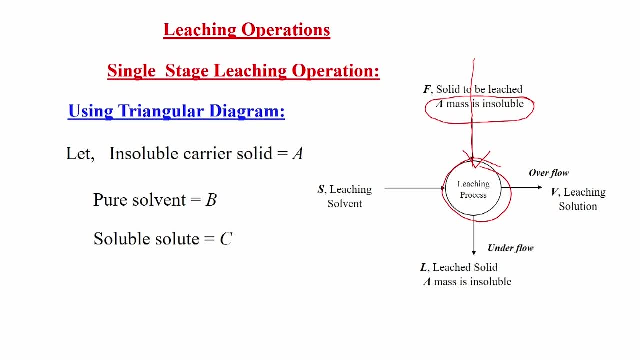 or we can say: this is nothing but this inert. so we can say this one insoluble, solid career that is in A, it is equivalent to that of the. we can say this carrier solvent, like that in case of this extraction A, and then pure solvent, whatever is added. that is, we can say this: 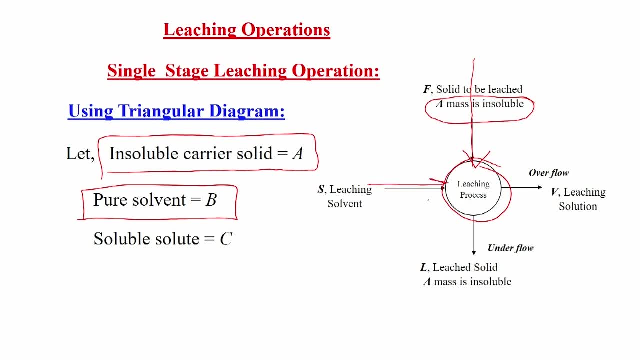 one B. so here we can say this: one pure solvent is added. so we can say this: one B, but we are adding this S amount of this pure solvent. we can say this is leaching solvent because it does the leaching process. leaching is nothing but coming out of this solute through. 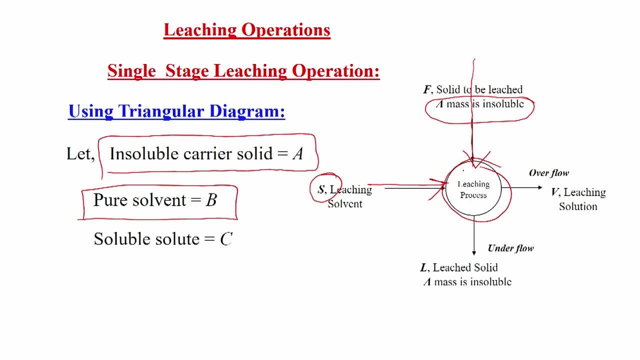 from the solid material. When we are allowing this process to reach its equilibrium, then it will be converted into two. we can say this: one phases, one will be the overflow, that is, we can say this: one that is our target. where we can say this overflow is V and one is this underflow, that is, we. 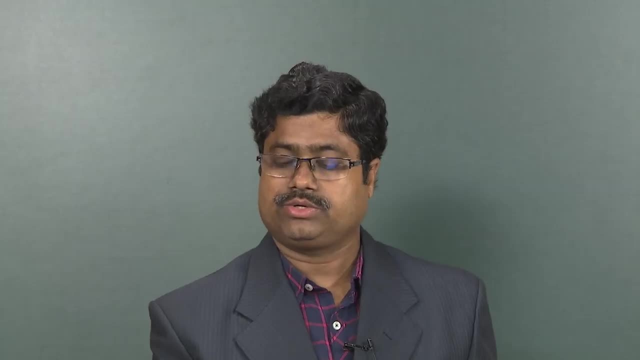 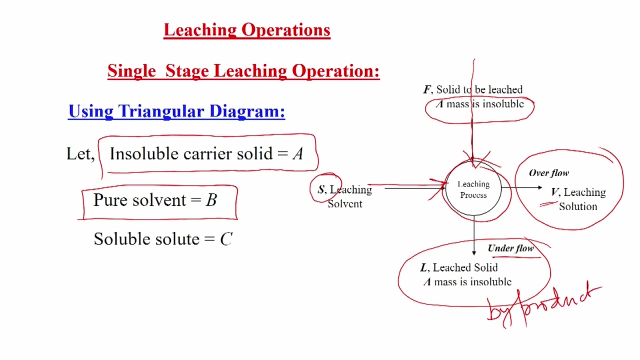 can say this one that is not required. or we can say this one: it will give this byproduct. so that is, we can say this one, that is, we can say underflow. or we can say this one: leached solid or exhausted solid. But we need to remember that the- whatever the target component C is there- say soluble. 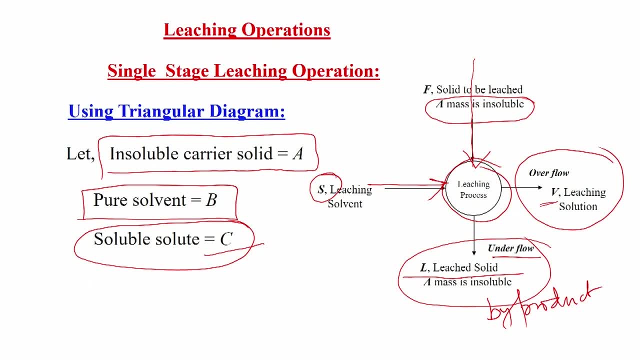 solute, or we can say this: one target component will be divided into two parts like this: one part, major part, will go to the- we can say overflow, and minor part will come to or will be carried through this inert, insoluble solid, or we can say this, one which is inert. 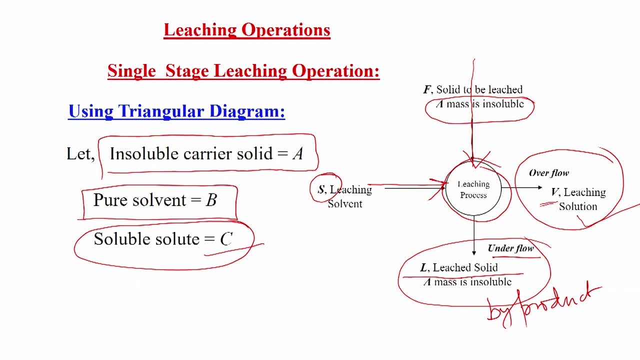 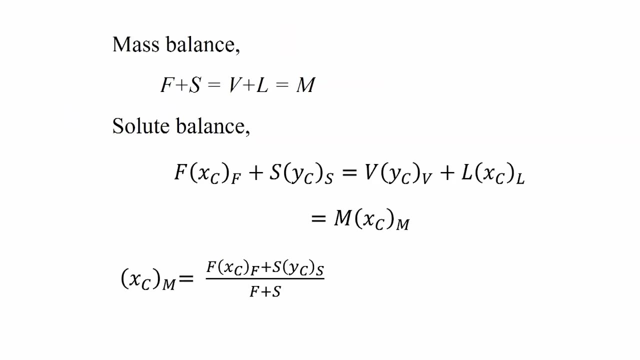 So we cannot completely remove this. we can say this target component, This one from this inert, because there will be some amount of association of this target component with the. we can say carrier solid A. So we will be doing this simple mass balance. that is very easy. they say feed plus solvent. 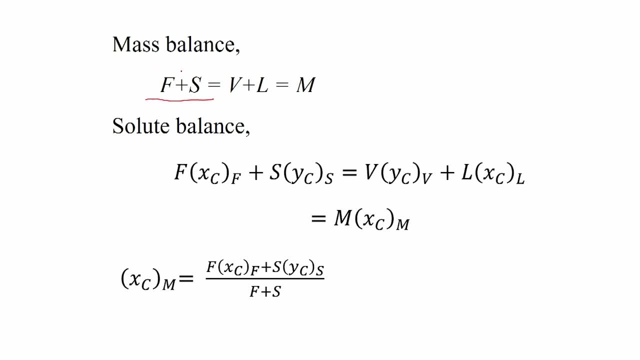 we can say: this one feed contains some amount of- we can say- inert material, and that is A amount of inert material plus, say, some amount of the solute And this solvent. that solvent may be free of the solute or may be sometimes it. solvent may contain some amount of the target component also, and then it is nothing but the summation. 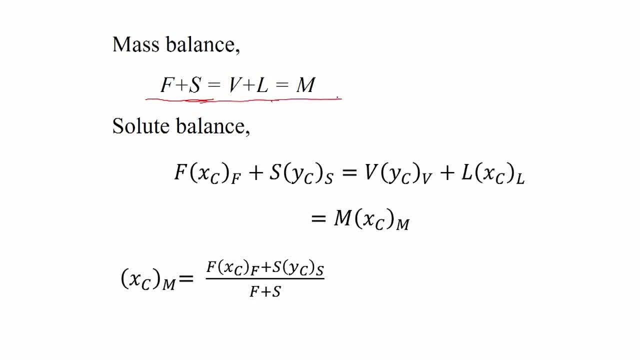 of this underflow and overflow. that is the mixture. So if we do the solute balance then we can say: F into Xcf, then how much amount of the this target component is there, plus this S into Ycs? sometimes it becomes 0. Why? 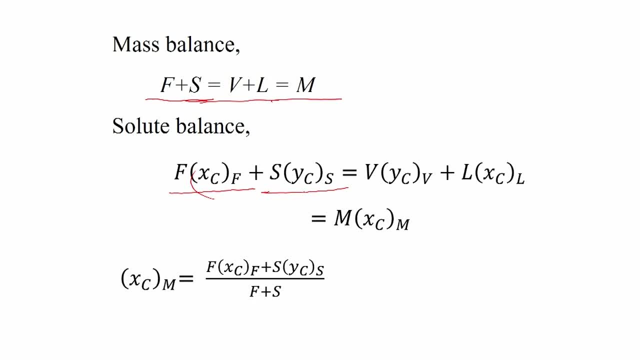 Because Ycs becomes 0 if it is pure solvent. if it is not pure solvent, then Ycs will have some values. Then it is nothing but this: V into Ycs plus L into Xcl. so this is nothing but M into Xcm. so this is this concentration of the solute in the mixture, that is, we can say this is: 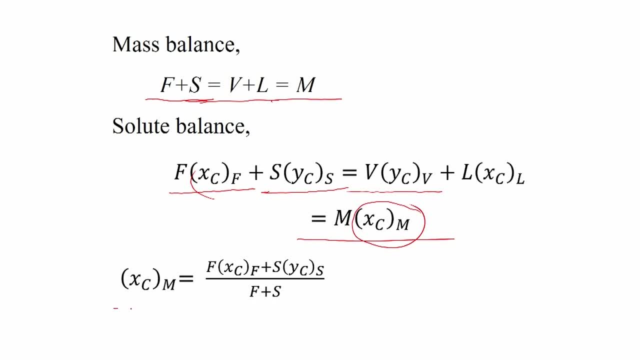 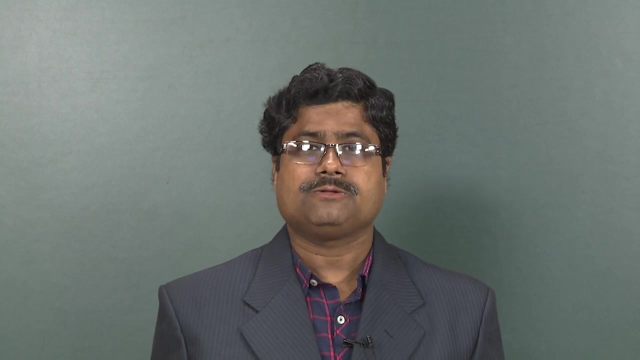 a fictitious concentration. So Xcm is nothing but the. we can say this one: F, Xcf plus S into Ycs, So we can get the solute concentration in the mixture. but in reality we cannot get this one, what is called concentration, because it will be separated into two different phases. 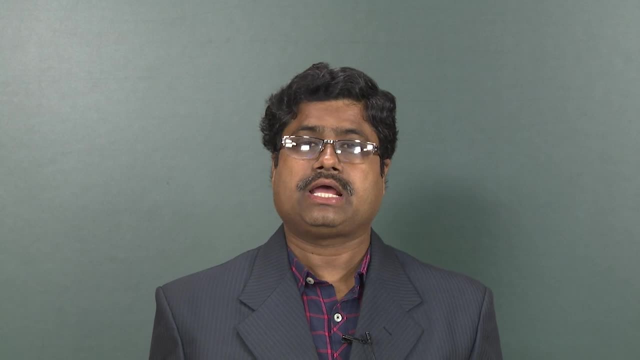 and we already we have mentioned that sufficient time is given for this- either extraction or leaching process to be separated into two different phases, like this: in case of this leaching, So we can say that is under flow and over flow in case of this extraction process, that 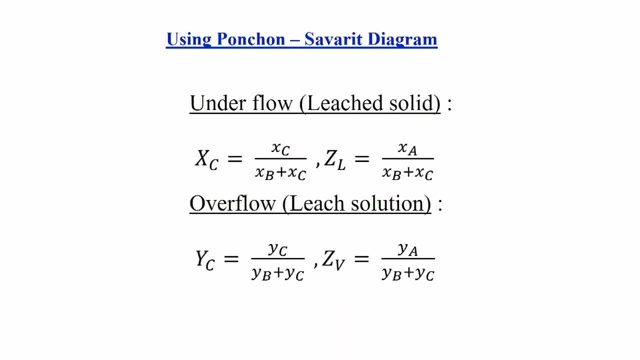 is. we can say this: extract and raffinate. So, using this Ponchon-Savary diagram, say now we are converting this one, all this, we can say this, we can say this: solid, free basis. so there, we can say this, under flow, that is. 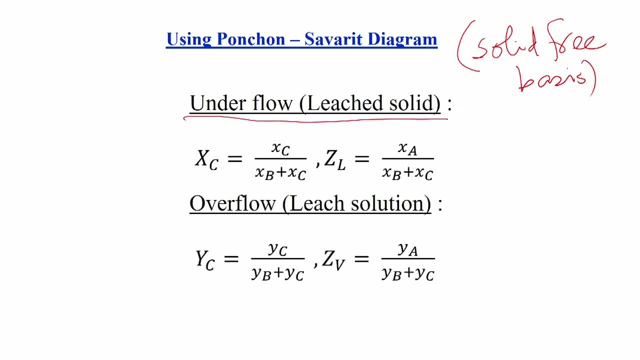 leached solid, or we can say this one: whatever the cake, or exhausted solid will be there, excess will be there, Exhausted solid. Exhausted solid XC will be XC by XB plus XC and ZL will be XA by XB plus XC in case of this under overflow. 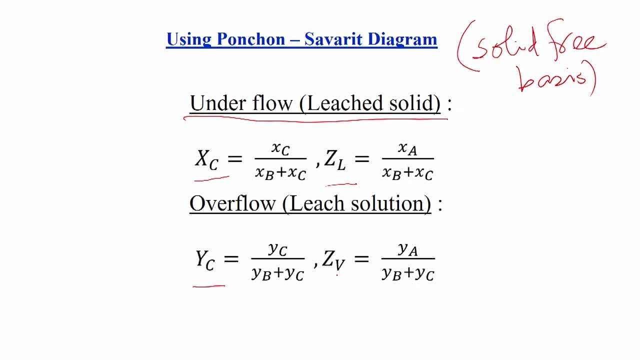 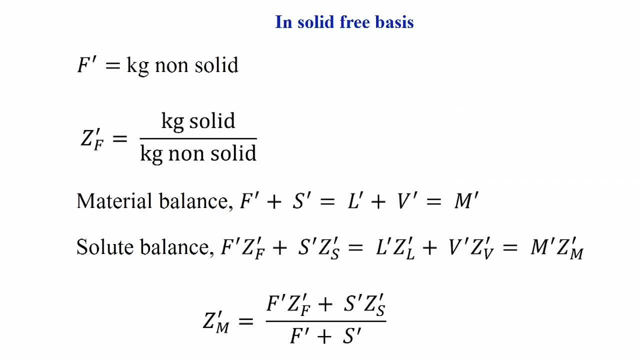 that is, YC is equal to YC by YB plus YC and ZV is equal to YA by YB plus YC. So these are the- we can say this- one solid free basis, or sometimes we do this one F prime or ZF prime. we use this one where this everything is the solid free basis, like this, all the. 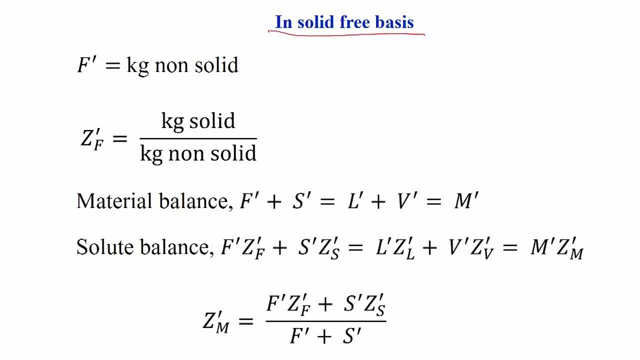 components. or we can say this: all the streams are solid. free basis means this: one feed extracting solvent. or we can say this: underflow, overflow, then it will be like this: ZF means say this: whatever the fraction of this we can say, this particular material, that is, will be in terms 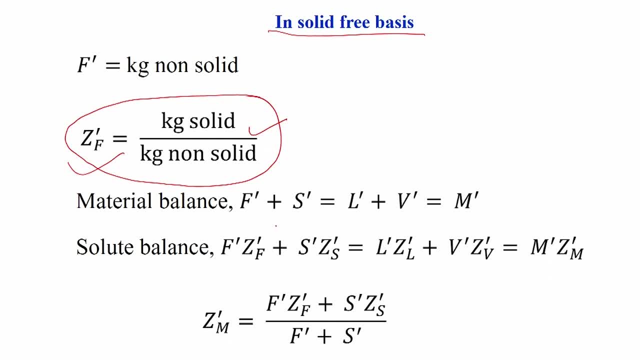 of kg solid by kg non-solid. So in that case we can say: the F prime will be kg non-solid means which is solubility only in the- we can say this one in that particular operating condition. so in that case we can say: F prime plus S prime will be L prime plus V prime. that is nothing but this M prime. 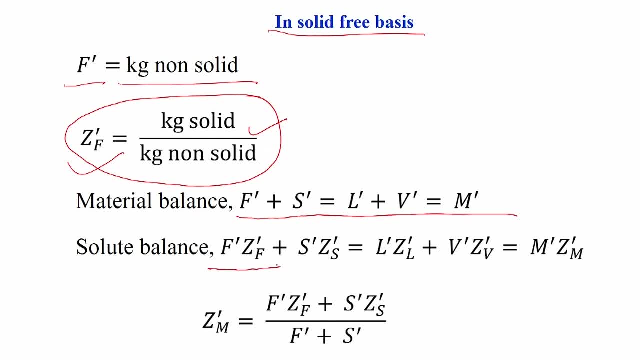 so if we do this solute balance also, that will be F prime into ZF prime plus S prime into ZS. prime is equal to L prime, ZL prime plus V prime, ZV prime is equal to M prime, ZM prime. from where we will be getting this ZM prime here? also the concentration of the 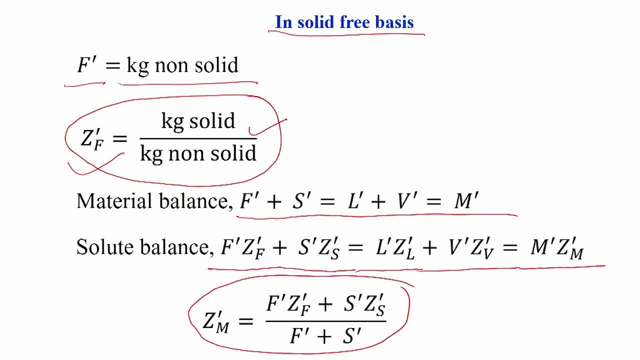 solute that is in. we can say this is solvent, solid, free basis. that will be nothing but this F prime, ZF prime plus S prime into ZS prime by F prime plus S prime. or we can say this: one will be in place of this F prime plus S prime will be L prime plus V prime. 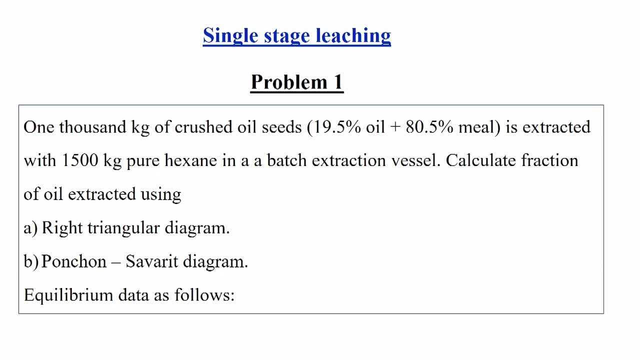 Now we will be solving simple problem for this single stage Leaching process. very simple problem and like 1000 kg of the crushed oil sheets, like here, 19.5 percent oil is there and 80.5 percent meal is there, or we can say this: peanut or 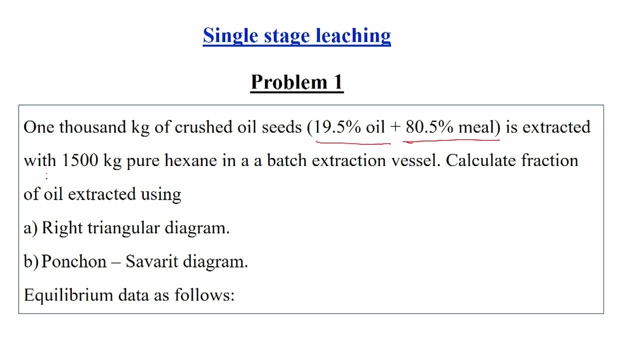 cake is there that should be extracted with 15000 kg pure hexane. so here you see. this solute concentration in the hexane is 0, in a batch extraction vessel. so we need to calculate the fraction of the oil extracted using this right triangular diagram and Ponchon Savary. 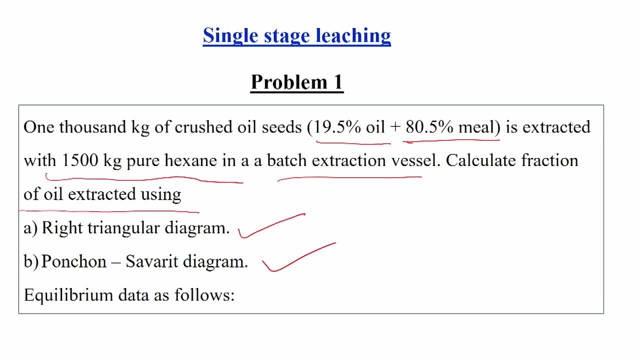 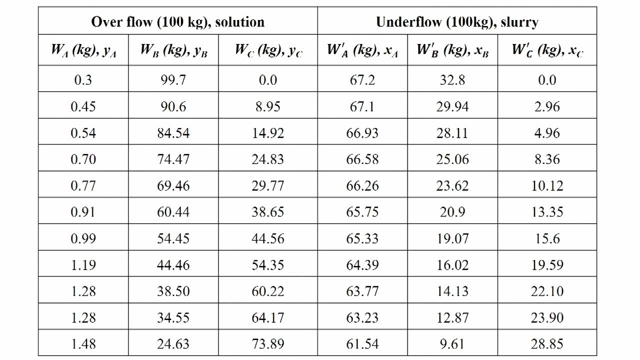 diagram For that, say, equilibrium data are given, like this one. so here you see this one. it is expressed in terms of 100 kg, but whenever we will be putting this one in either of this, we can say: right triangular diagram or Ponchon Savary, we need to convert this into the corresponding. 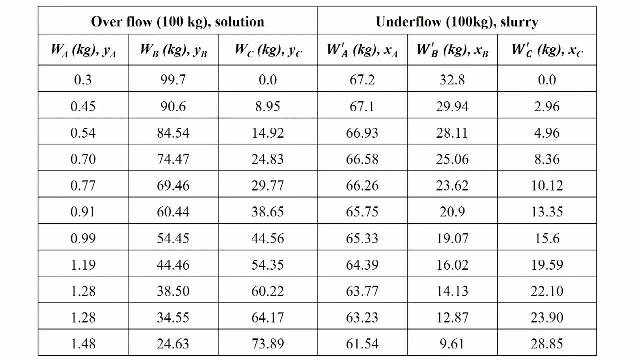 we can say this one: YB, YC, Okay So YC or capital, YC, capital YB, and with this one we can say this one: so now it is in the suppose in terms of 100 kg, so we need to convert this into this. we can say this: fraction. 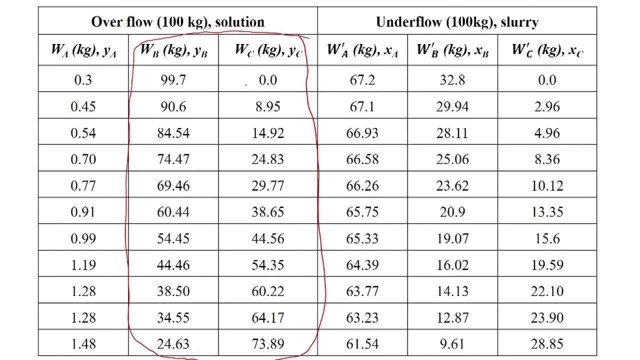 like this: YB will be 0.997 and YC will be 0, and that way we can say this one this: whenever YB is equal to 0.2463, that time this YB will be 0.997.. Okay. 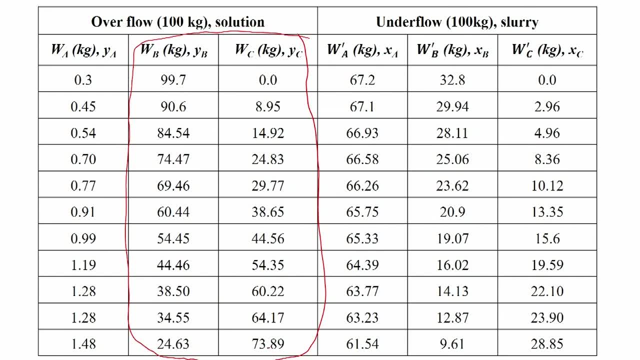 Okay, Okay, So this YC will be 0.7389.. So we need to remember this one also whenever we will be drawing the equilibrium diagram, say in the ternary diagram, we need to convert this one. for this we can say whenever we will. 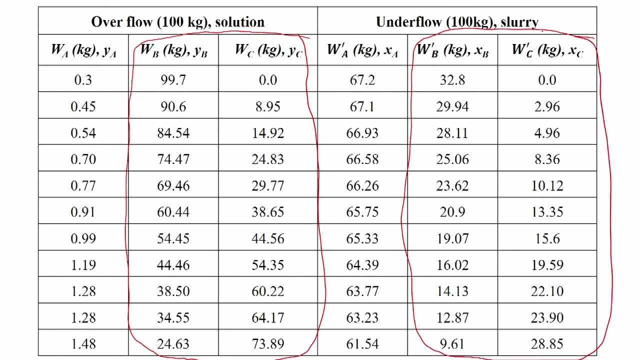 be putting this one in right triangular diagram, we need to convert this into the fractions only, Okay, And whenever we will be putting this one in the Ponchon Savary, then we need to convert this one in the solid free basis. Okay. So that is very crucial one, but remember that whenever this type of correlations are given, 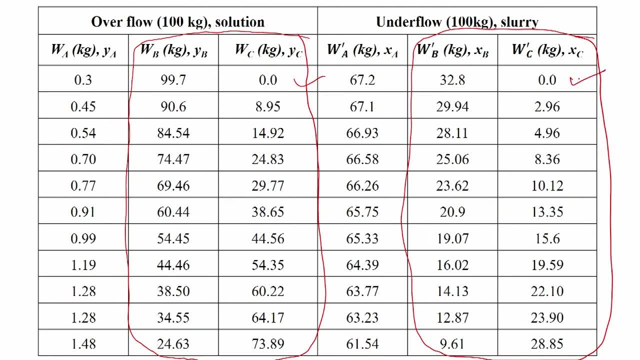 then we can say this one: this YC is in equilibrium with this YC and this YC is in equilibrium with this YC. So this is, we can say this one, this YC and XC, these are also equilibrium data points. or we can say this: tie rhyme values. and one interesting point that already I mentioned: 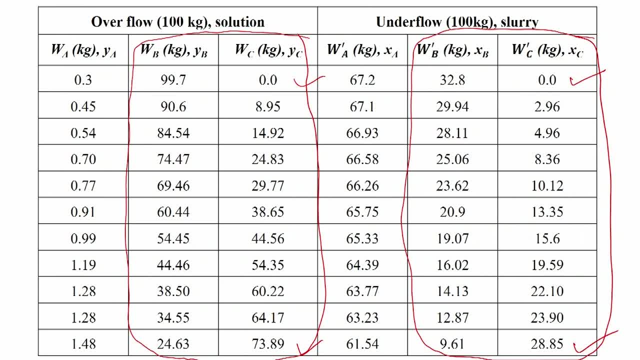 that in case of this solid liquid extraction, whatever the YC and XC values are there, they are there, It will cross this. we can say this: 0, 0 point, okay. So that is this one. that is one advantage of this leaching process and we will be discussing. 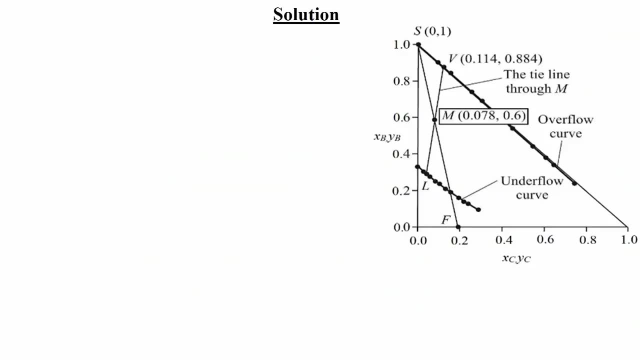 this also in this problem also we will be discussing. okay, So we will start solving this one. whatever the- we can say- data points are given already. we will be first using those and then we will be placing all these in the right triangular diagram. First we will strive this right triangular diagram. 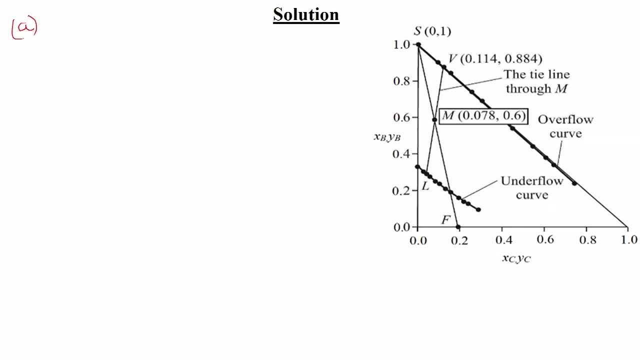 Then we will be doing this. Okay, So we will be using this one for the ponchon sourit. or we can say this solid, free basis will be this one doing that. So for this, whatever the data points are there already, we will need to get this one. say first: 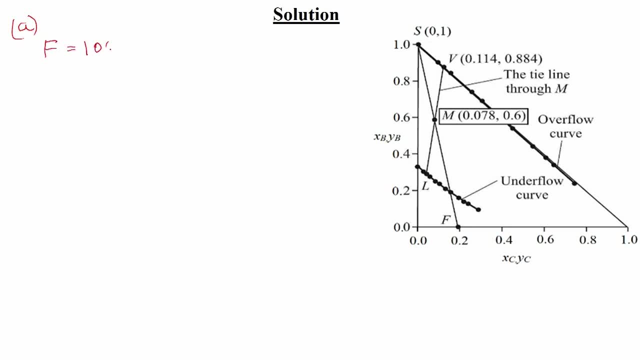 feed is given as, say 1000 kg and this solvent is given as 1500 kg. And then XCF, Okay, That is given as say 19.5 percent, so that will be 0.195. and where have this YCS that? 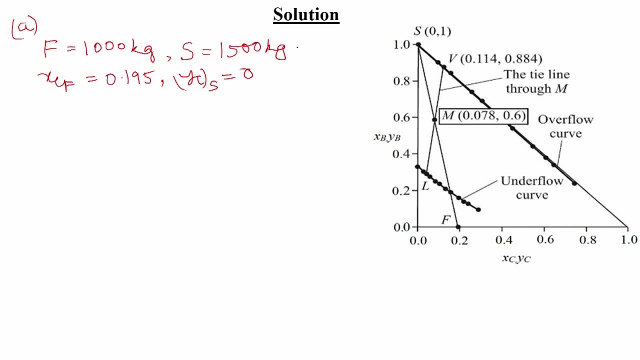 is. in that case it is 0.. Because it is a pure hexane is given, so it is. it has no contribution in the towards this. we can say: this oil extraction, okay, So we have this now. mixture is equal to, we can say F plus S, that is will be like 2.5. 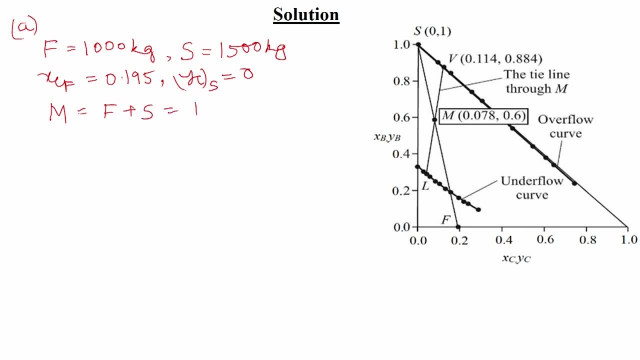 Okay, Okay, Okay, Now we can get this. say XC. say we can say this one M, that will be like F, XCF plus S. say YCS by F plus S, So it is coming out as 1000 into 0.5.. 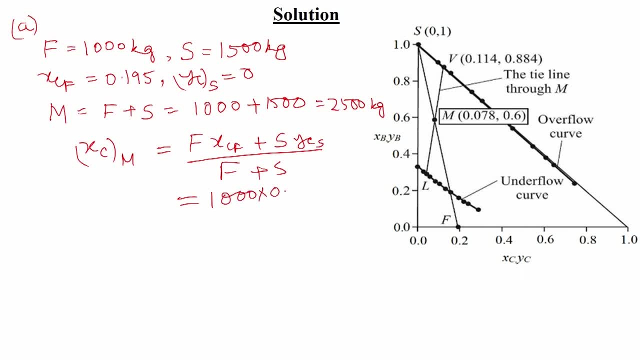 Okay, Okay. So it is coming out as 0.5 into 0.195 plus 1500, into 0 divided by 1000 plus 1500. So it is coming out as very small value: 0.078.. So we will be now getting this, three points like this. so first we need to locate, so first, 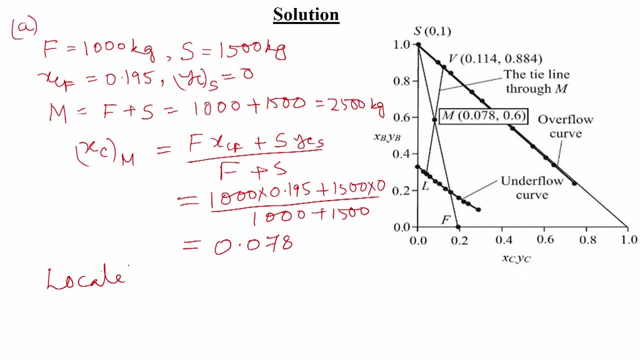 step will be locate This F, that is, we can say this one F will be like this: in the C axis. So every time, actually, we put this one F in the C axis because it contains only A and C. okay, So there is no B, okay. 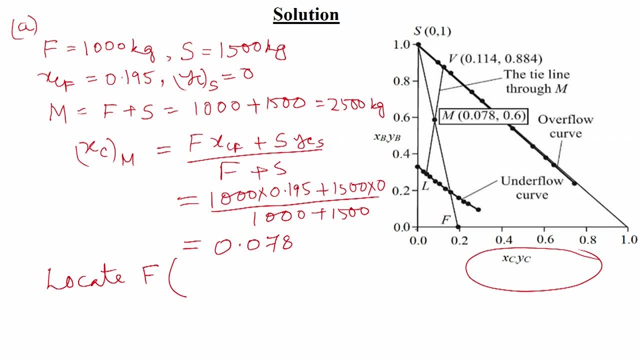 So, because you see A is the- we can say this inert- and or we can say this one carrier solid, and C is this, we can say Okay, We can say this one target component, So it is, we can say this one: 19.5.. 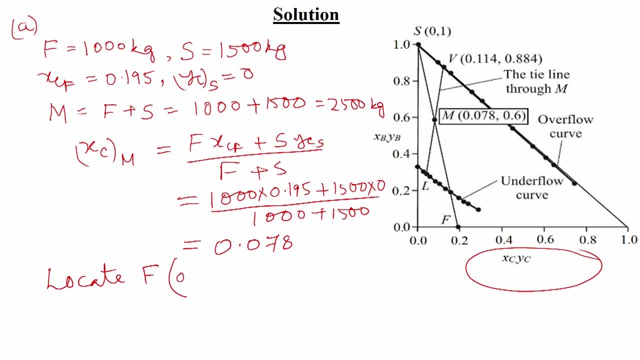 So we can say: F will be like this: 0.195, almost this one here, with this YB, that is equal to 0.. So this is coming out here, Okay. And then we have this S for S we can say this one XC is 0 or YC, whatever is that is 0, and 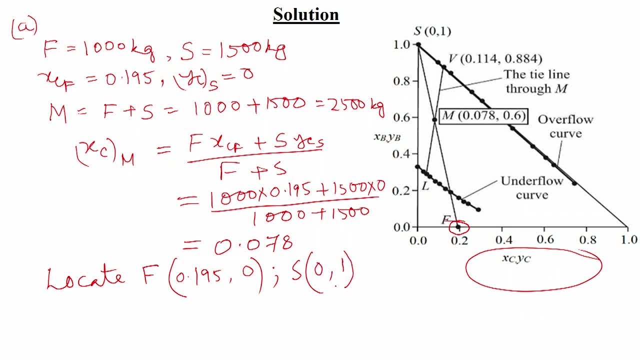 the as this is a pure one. So we can say this: one YB is well done. Okay, This is equal to 1.. So this is nothing but this point. Okay, First we need to join this S and F. I am not repeating the. we can say procedure or we can. 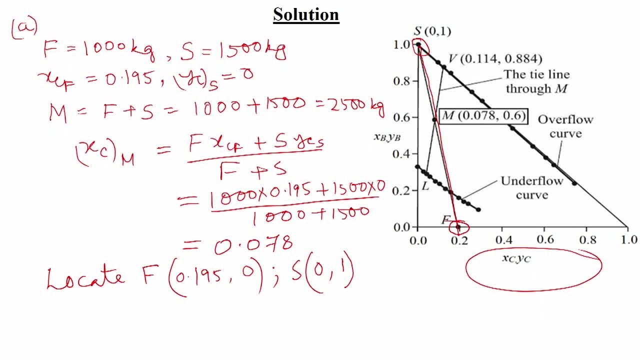 say this: one design calculation for this leaching unit, because this is the same as we followed in case of this liquid extraction, So the same procedure actually we need to follow. So we need to join this S and F and now we have this XCM, that is, we can say this one. 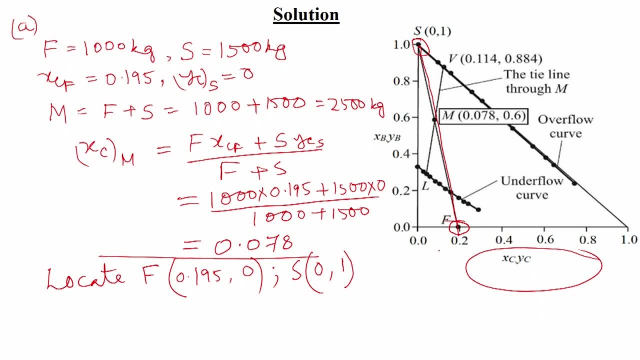 0.078.. So somewhere it will be like this one, So this one, 0.078.. So we will be coming to this point. say, that is, we can say this one XC is equal to 0.078. So then we will be getting this M. So now we have this S and M is like this: a mixture. 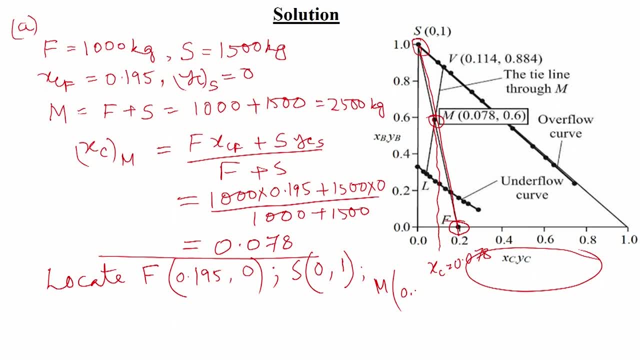 point. It will be like this: 0.078, and from here actually we will be getting as this around: say, Y will be like 0.6.. So it is like here. So we are getting this M here. So that is placing in this line. 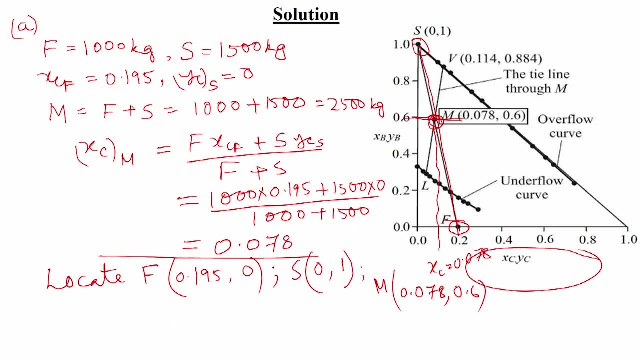 Now the procedure is very simple, like this one: Whenever we have this M. I mentioned that if we just draw a straight line from this 0.0 point, So then it will be like this: if we start from here and if we extend this one through M will. 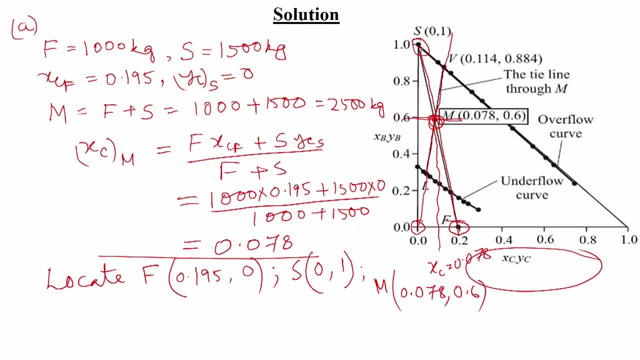 be get it will touch. this. we can say: this overflow line and this underflow line, It will touch. this means if we keep this mixture for a long period of time, then it will be converting into 0.078.. This, we can say this: one underflow and overflow. 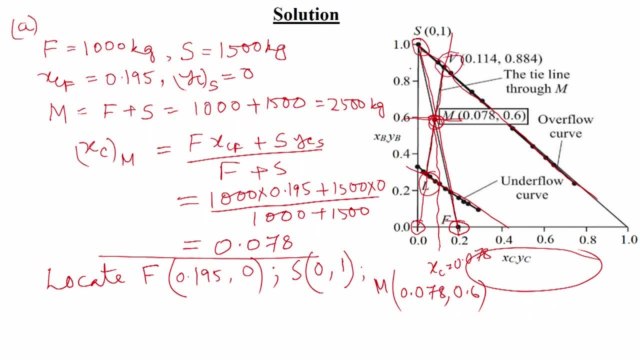 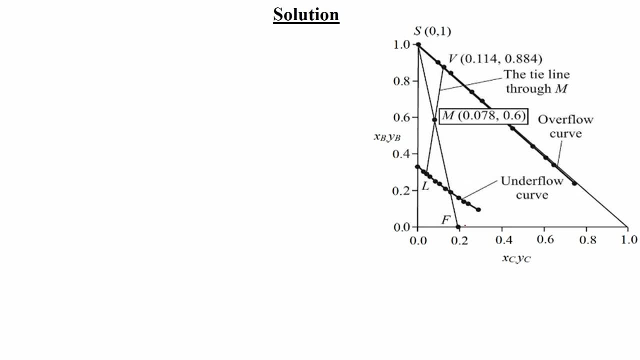 This overflow line means it will be touching at V. So we can say this one, say we have this now. we can say this one: it is converting. now we have this F, we have we have S and we have this. we can say this one mixture. 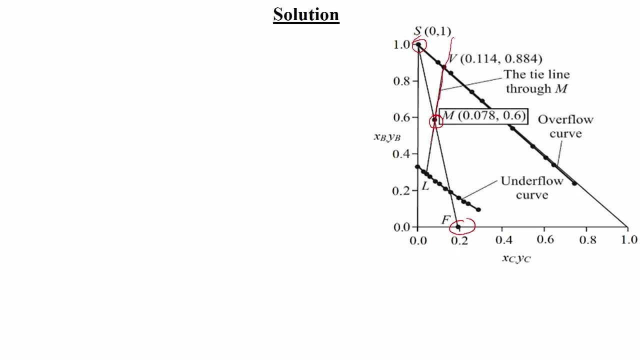 Now we are drawing this straight line. that is nothing, but that we say: I told that this is the tie line for this one, and now it is converting into V and L, So So here this from this diagram actually will be getting all this composition like this: 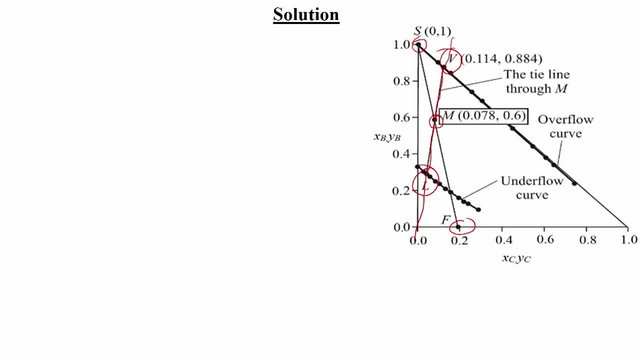 so here we can say this one: if we do the component balance here, say like this: say we can say this one V into say YCV. plus we can say this one L into say XCL, that will be nothing but say M into XCM. so here this mixture is, here actually we say 2500, so now we can do one. 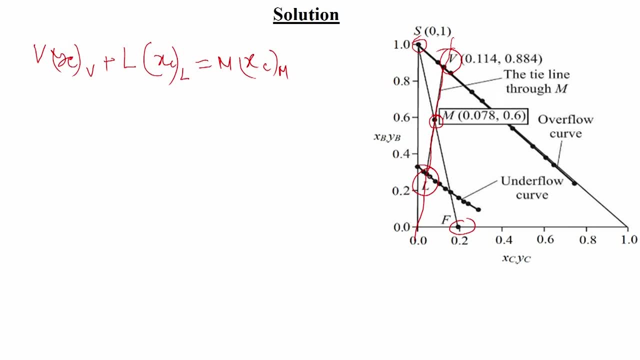 thing say from here, and so whenever we will be using this graph paper, we will find that the for this L, this. we can say we will be getting like this from this graph. or we can say right here from the graph, So say YC will be like this: this value actually is 0.114 and XC that is obtained as XC you. 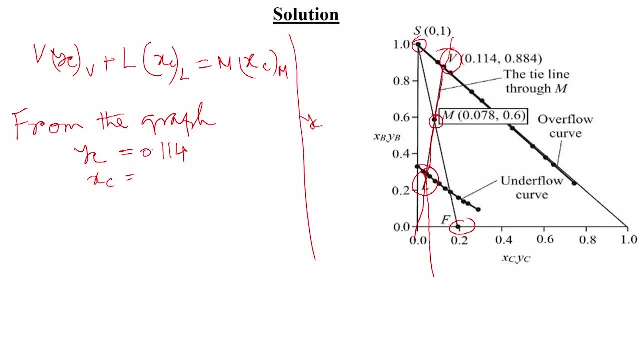 see this. sorry, this V into YC, this one that is obtained as 0.114 and XC will be like this one that is 0.114 and for XC it is obtained as 0.0403, so this is, we can say, this one, 0.0403,. 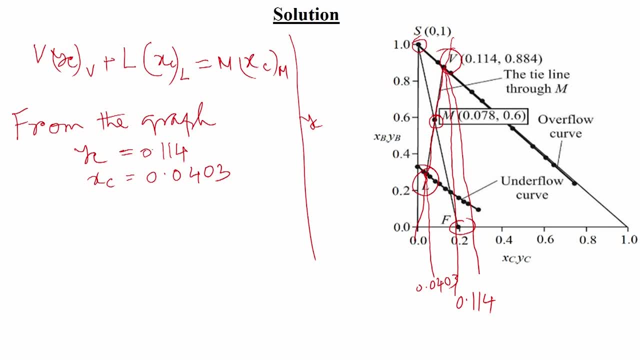 so will be this one. getting this one from this graph paper will be easily getting this one, and now will be putting this one in the. we can say this one in the component balance from where will be getting this one? So we will be getting both L and V, so we will be putting that V into YC. that is nothing. 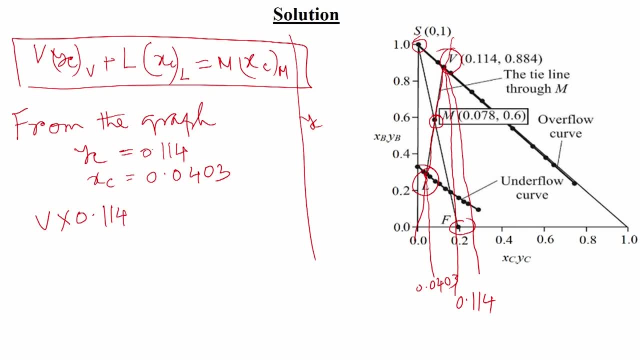 but 0.114, that is. we can say this: that is in the overflow line plus L into 0.0403. that is equivalent to 2500. that is, the mixture into XCM is obtained as 0.078, 0.0403. that 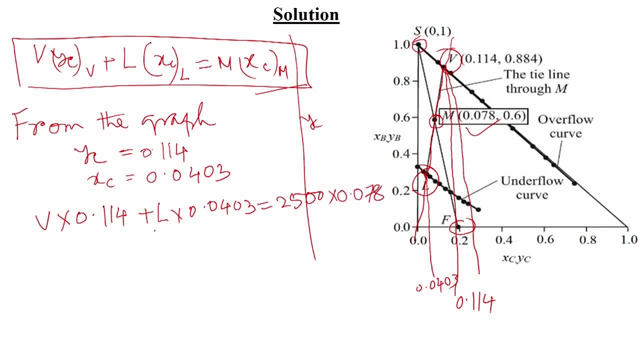 is 0.078 and we know this L is equal to. we can say this one: 2500 minus V, that is L is equal to 2500 minus V. So will be: putting now say V into 0.114 plus 2500 into 0.0403 is equal to say 2500 into. 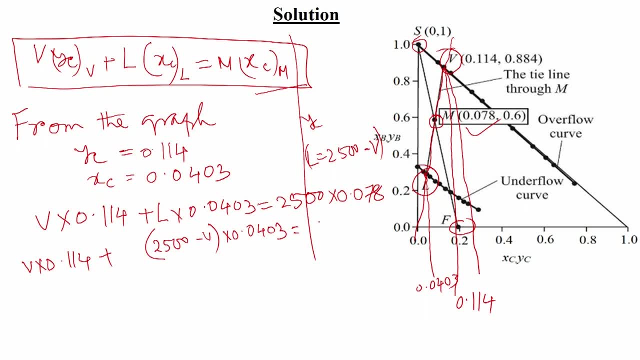 0.078.. So that is coming out as we can say 195,. so from here will be getting: V is equal to 1279 kg and say L is equal to, we can say 2500 minus 1279, so it is coming out as 1221 kg. 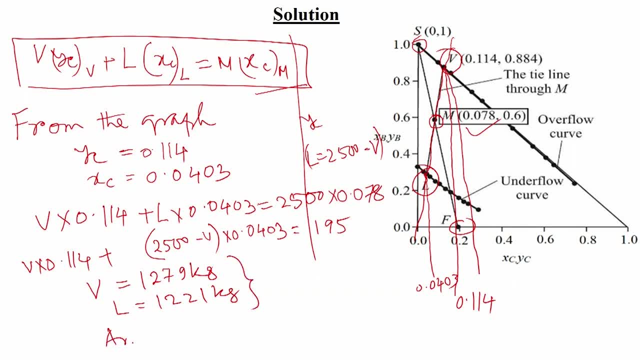 so now so the amount of- we can say this one amount- tasks of oil, we can say this one, extracted, that is, we can say this one: V into YC. V that is coming out as V is equal to 1279, into YC is already obtained from this graph that. 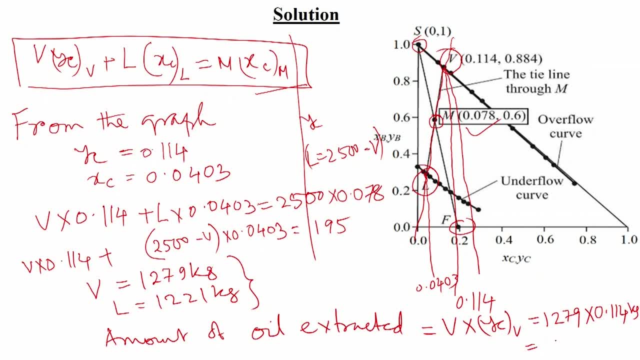 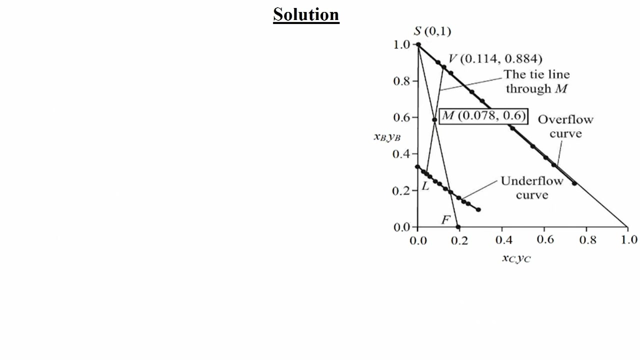 is 0.114 kg, So it is coming out as 145.8 kg. so now we have this dash amount, this 145.8 kg oil in the overflow. so from here you can say this one, the fractional, we can say this one extraction. 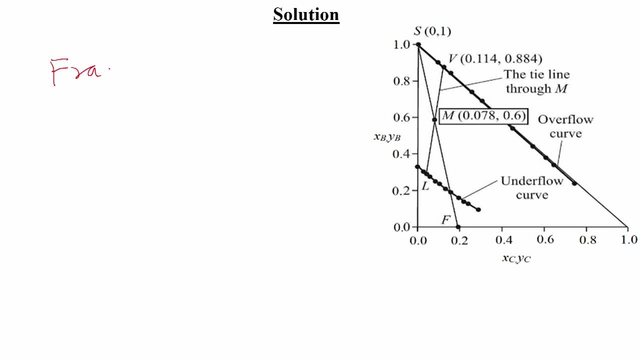 or we can say this: one fraction of oil extracted is equal to. we can say this: one total oil was actually say: we can say this: out of 1000 kg say 19.5 percent, that is nothing but 195 kg. So out of this 195 kg, that 145.8 kg is extracted. 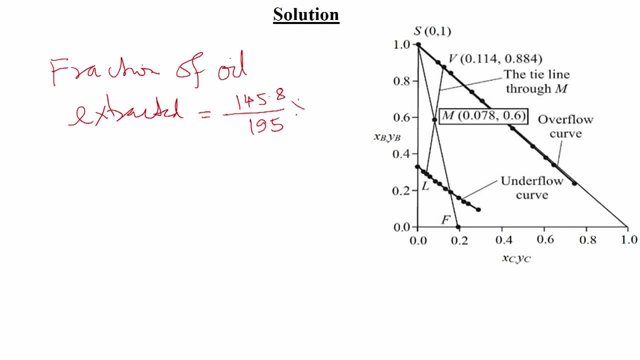 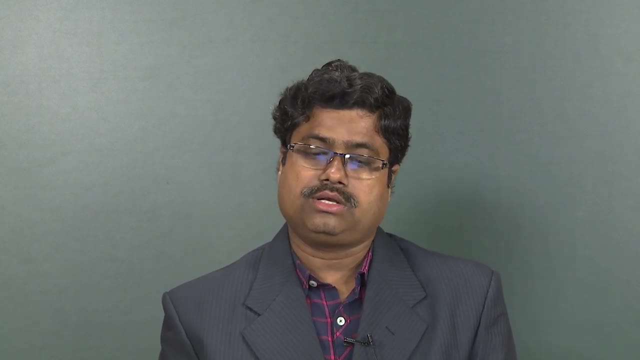 We can say this one recovered, or we can say extracted, so we can say this one percentage, so it is coming out as 74.8 percent. so using this single stage operation, this 74.8 percent oil is extracted from the. we can say this one extraction, this leaching unit, so there, 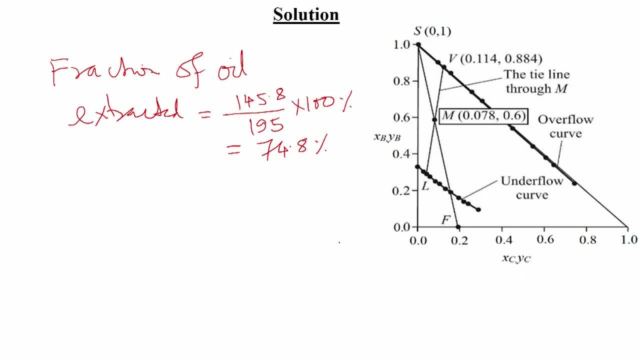 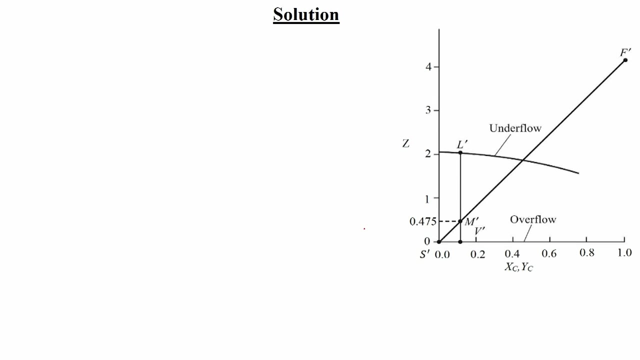 15000 kg hexane is used for the separation of the oil. Now we will be discussing with the using this Ponchon-Savary diagram. so I told that say whenever we will be this one solving this problem using this Ponchon-Savary. this is 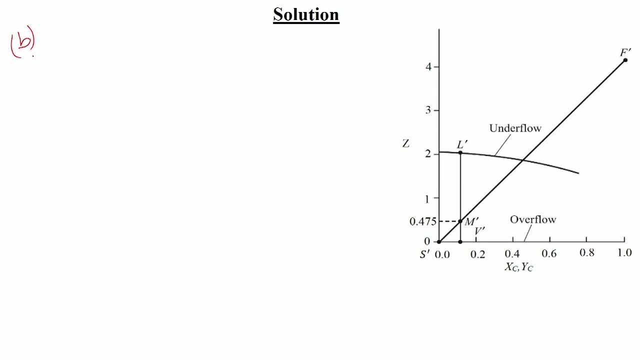 the second, we can say this one way of this one solving the problem. So there, we will be converting this overflow and underflow in terms of we can say this one: capital A, Okay, Capital XC, capital YC. and we can say this one Z, so Z values. so we will be getting. 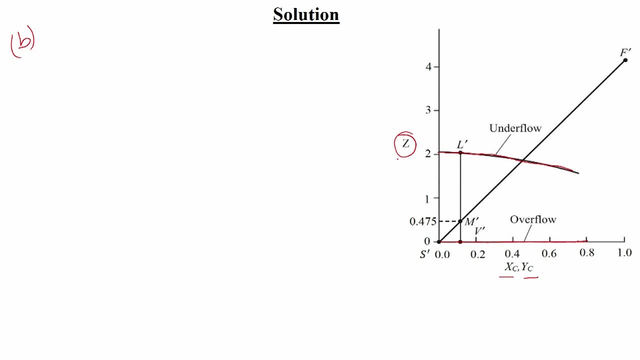 this one. so now ZL and ZV. so we will be putting this one and then we will be getting the underflow and overflow line. and I told that this, in case of the underflow, the, in most of the cases the values will be more than 1, okay. 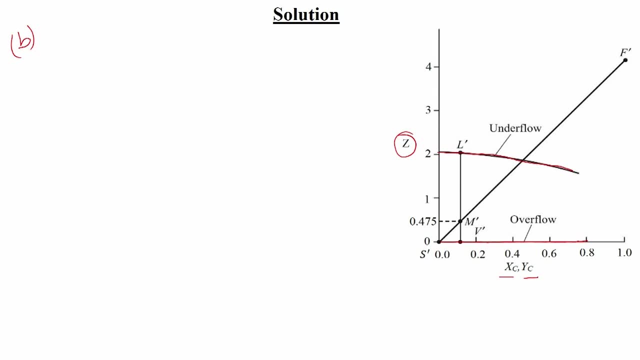 So that is, we can say this one: mostly it is the inert material. so we can say this one: where the KX will be there or we exhaust solid will be there And this F prime, whatever the feed actually has this, we can say this Z value as more than 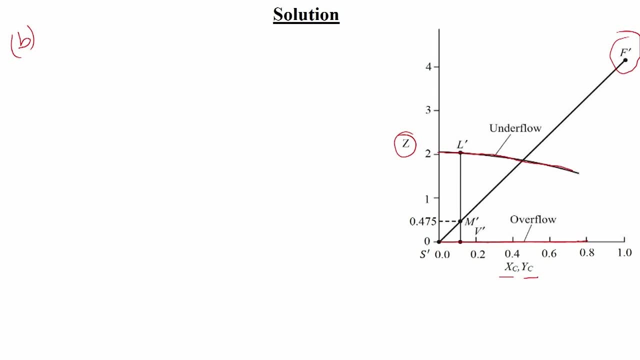 this one, what is called 4 here in that particular case. okay, So now here we will be doing this one in terms of this solid, free basis like this F prime will be like this: so out of this we can say this one, whatever the, if we this, we can say: 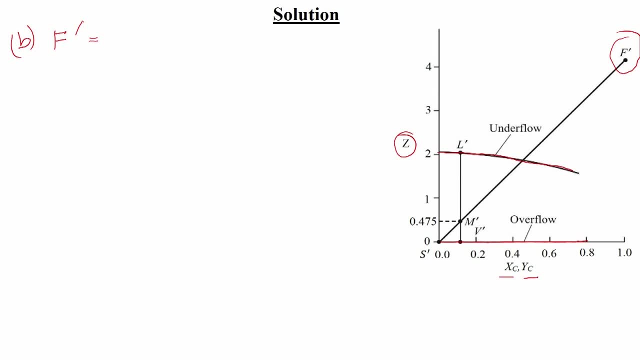 this one. if we remove this inert solids- Okay, So we can say this one: only 90.5 percent solubilized solid is there. then it will be like this: 1000 into 0.195. that is, we can say this one: it will be 195 kg. 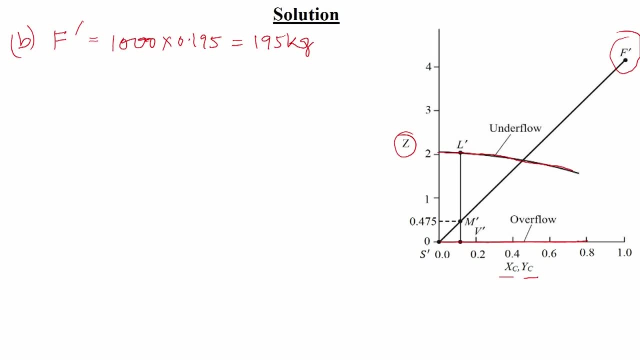 So this is: we can say this F prime is the 195 kg, that is. we can say this one: it is simply nothing but kg non-solid. okay, So this is called kg non-solid, Okay. So if we say Xc F prime, actually that will be like this: we can say this: one mass fraction. 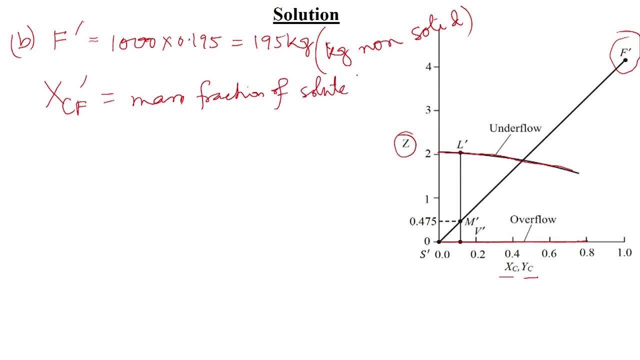 of solute, so in feed. So that will be. we can say this one: wherever it is solute in feed, and that is also in non-solid basis, we can say this one. so it will be like this: 195 by 195.. So that is nothing. 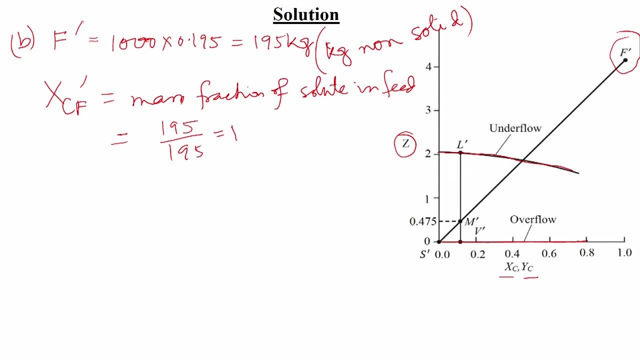 Okay, So that is nothing but say 1, because you see this in total solubilized solid. so how much amount of this one target component is there? so that is 195 by 195.. So whenever we will be discussing Xc, F, that is, in all the cases, it will be like 1, okay. 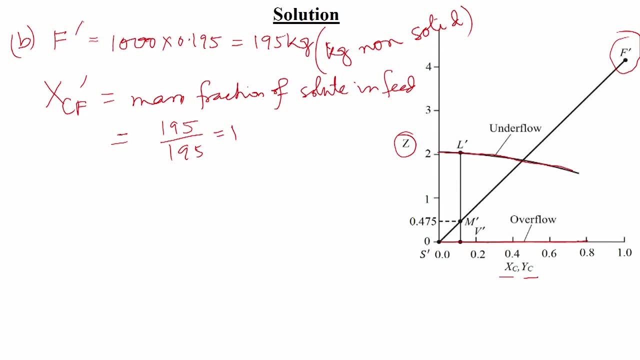 So Xc F, that is, we can say this one that will be always like 1, okay, Xc F. And then say Z F prime actually, so that we can say this one that we derived as 0.195. Okay, Okay. 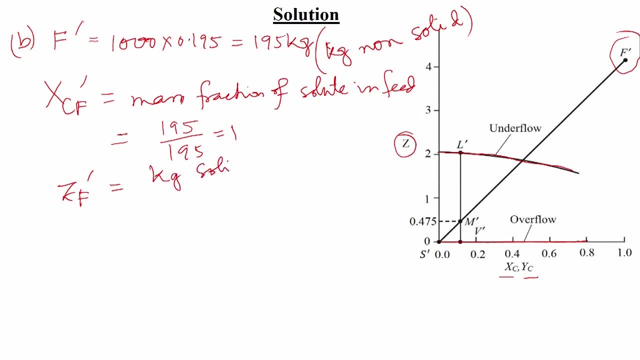 So that is derived as kg solute by kg non-solute. So that is the convention. So this here actually kg solute is, means this: out of this 1000 kg, 195 kg is the kg non-solute, So it is. we can say this one, 1000 minus 195, that is coming out at 805.. 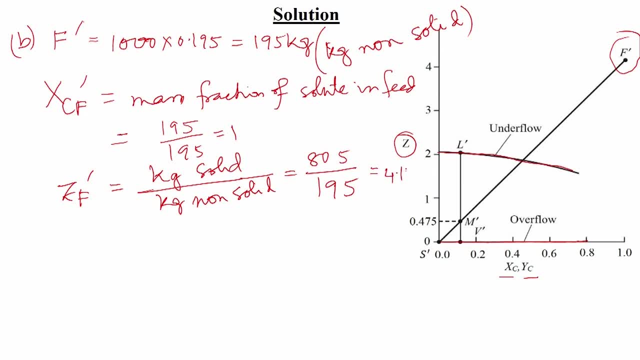 So it is coming out as we can say 4.13.. That is why you see Z F prime. Okay, So whenever, say, the value Z value of this feed is more than 4, so in that case, So as we have this one, so this is 4.13. so that is we can say this one and for this, whenever, 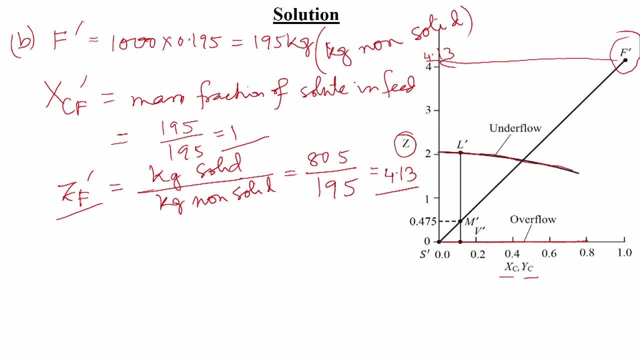 we can say, we can say this one: when Xc, F is equal to 1, or say capital Xc or Yc, whatever that is, for this case that is 1.. So this is, we can say this one feed point location is placed here. 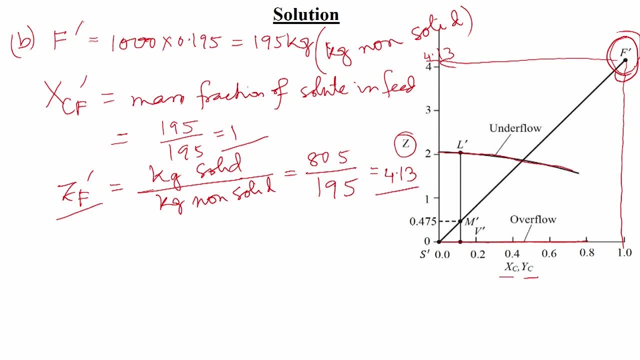 So feed point location is placed here now. Now we can say this Yc S prime. that is here. you see, this one, the same problem here, solvent is pure hexane. So it is. we can say this one is equal, to say Yc S prime, that is 0, and again say Zs prime. 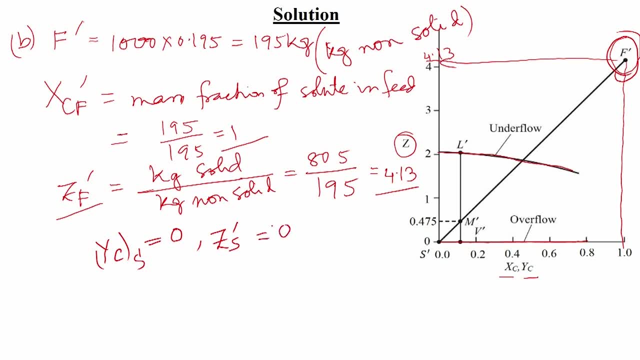 also that will be 0.. So because here this non-solid means that is target component that is not present in the Okay Okay, Okay, Okay, Okay Okay. Now this M prime will be like this: we can say total, we can say this one: the mixture. 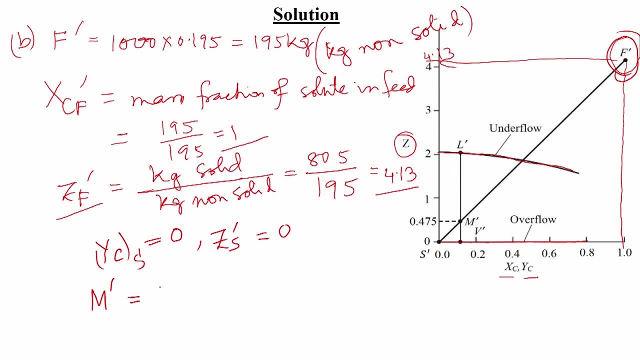 that will be in the solid free basis from this feed will be getting, say, 195 kg and this from the extracting solvent will be getting the entire one, 1500, because this is the pure, we can say this one non-solid, or we can say the solvent, so it is coming out at 1695 kg. 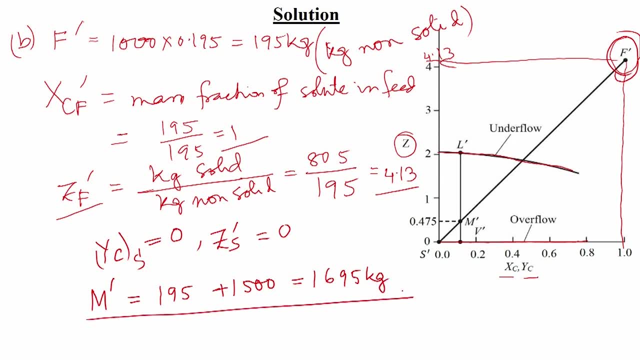 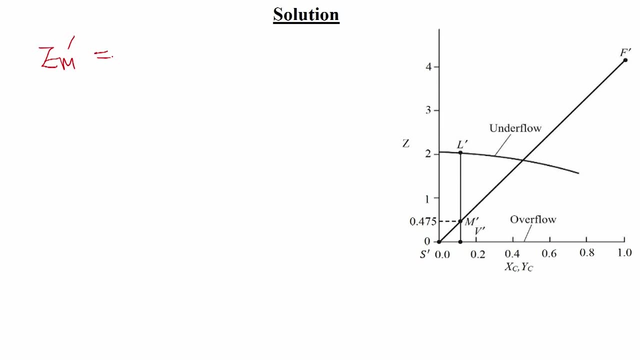 Okay, So total mixture is like this. So now we will be say we will be calculating this Zm prime. So Zm prime is nothing but this. from the formula we can say this: one F prime and Zf prime, plus we can say this: one S prime into Zs prime by this F prime plus S prime. 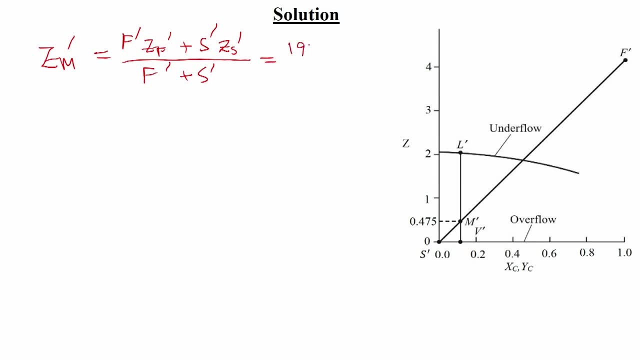 Okay, So it will be like this: F prime is 195 into Zf prime, into Zs prime, Okay, Okay. Okay. So F prime is, whatever we got this one, 4.13 plus S prime, that is you can say 1500 into. 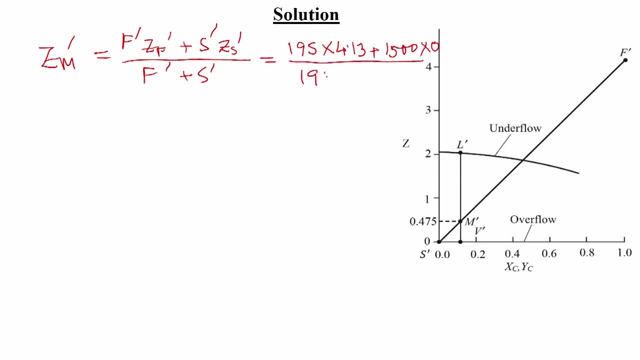 Zs prime is equal to 0 divided by 195 plus 1500.. Okay, So it is coming out as 0.475.. So you see this one in this case, whatever the mixture is there. Okay, So we have now located this feed point, we have located this S prime. that is nothing. 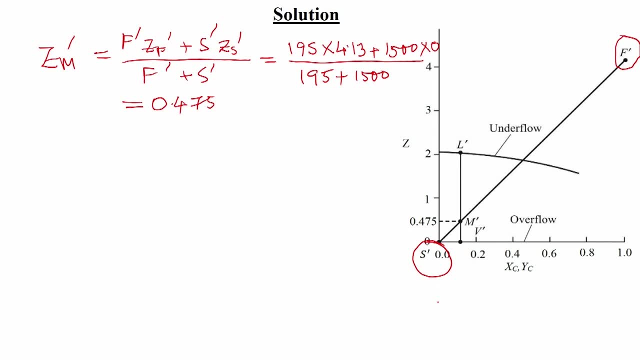 but 00 because it does not contain any. we can say this: one target component, Okay. So now again we need to join this F prime and S prime, as usual. then we need to get whatever the Zm prime is this one, 0.475.. 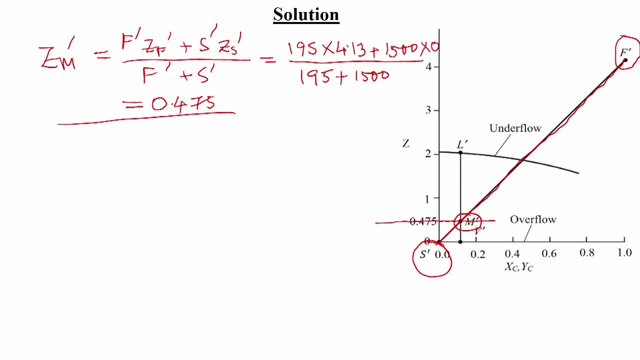 So for that case, we will be getting M prime here. Okay, And say this one, say M prime will be obtained when Z prime will be 0.475, like this: these are actually Z prime Now. you see this: F is located, then S prime is located and M prime is located. 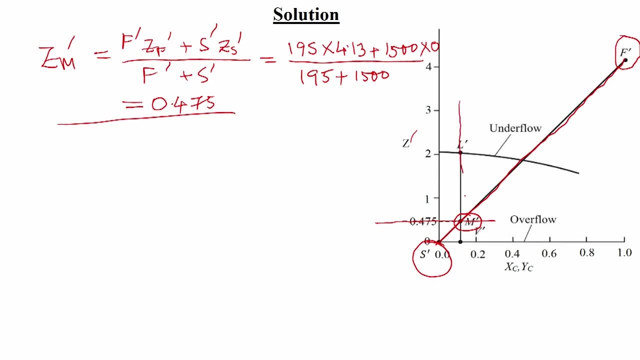 Now you see this one: all the tie line values are actually now vertical. whatever the tie line values actually we will be getting here, all will be vertical, because here we have- we are expressing this, we can say- all the underflow and overflow with the solid free basis. that is why all the tie lines are vertical. 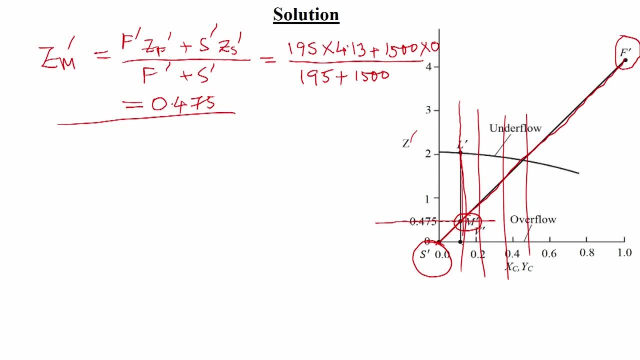 Okay, So now we need to this one, draw this vertical line through M prime that is lying in between S prime and F prime. Okay, So then we will be getting this L prime and we can say: this one will be getting here this V prime. 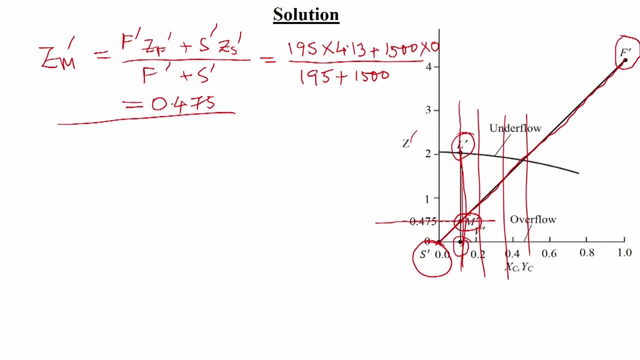 Okay, So we will be this one. now we will be getting this V prime and L prime. Okay, So there, actually we will be getting this Z L prime. that will- that is actually is just above this 2 that is obtained from this graph. actually it is obtained as 2.03 and say Z. 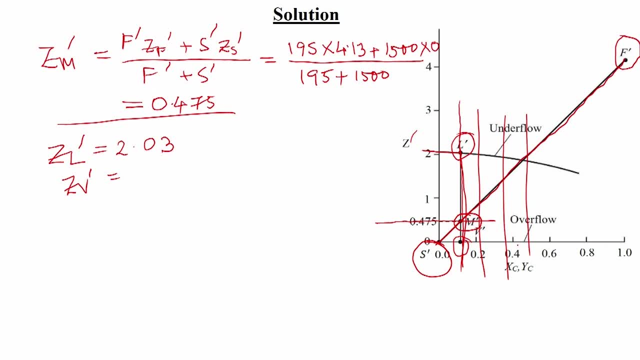 V prime. there is obvious that it will be almost 0 because you see this overflow line, whenever we will be converting this into, we can say this: one solid free basis in the overflow, because there will be no solid, there will be no solid. that is why it is we can say this: 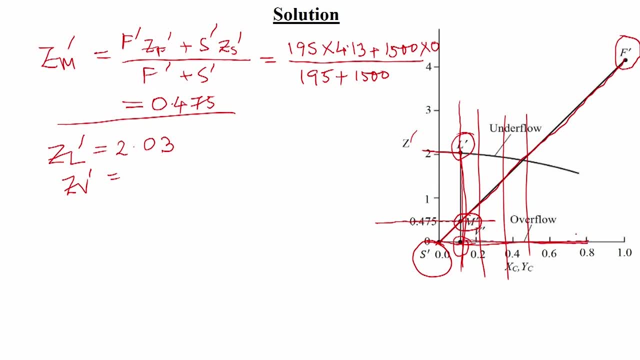 always it will be lying in the- we can say this one- X axis. So that is why Z V prime will be 0.. Okay, Now we will be doing this. one. say we can say this: X, C, M, whatever the values, actually we are getting this X C value actually followed. 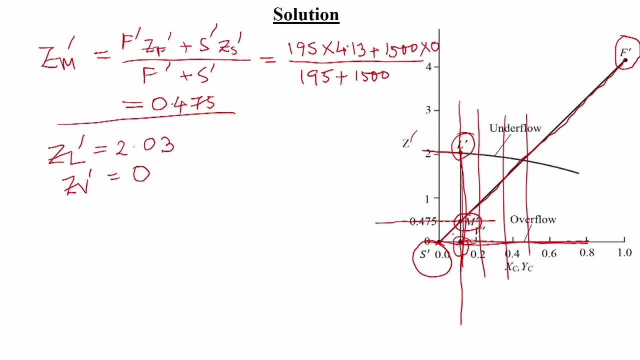 Okay, For this, that is for all the cases, we can say this: one for underflow, for overflow, for the mixture, that is X C M Z value, that is, you can say this: capital X C M value is nothing, but the X C L prime, that is nothing. but we can say this: one: Y C V prime, that is coming. 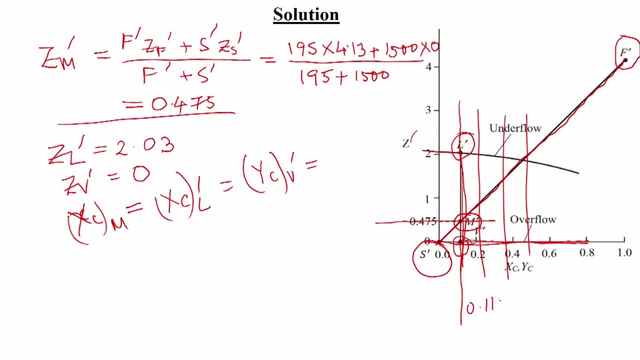 out as this one. this is 0.115.. So it will be. if we use this graph paper, then we will be getting this Y prime as 0.115.. So this is, we can say 0.115.. So now we will be doing again. we will be doing this component balance like this. we will be: 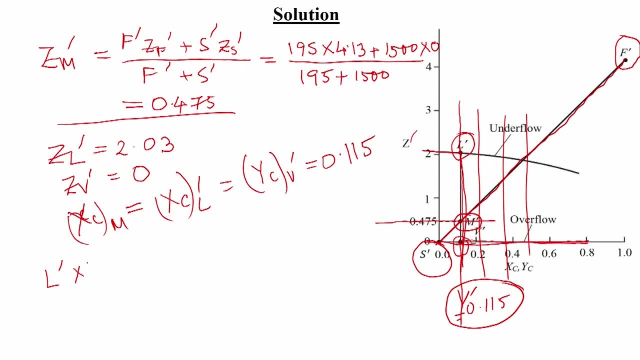 getting L prime into. we can say this: Z L prime plus V prime into Z V prime that will be coming as M prime into Z V prime. Okay, So here this one. we can say this one L prime into Z L prime that is coming out as Z L prime. 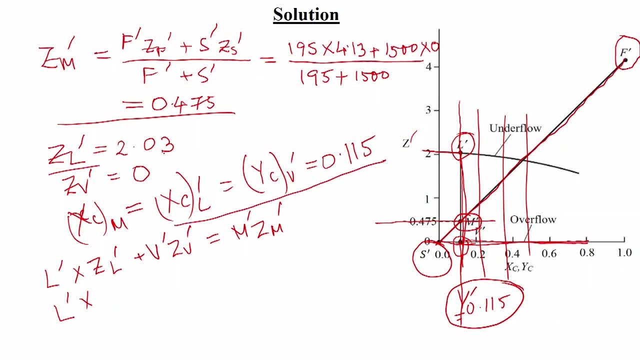 that is we can say Z L prime 2.03.. So that is 2.03 plus V prime into Z V prime. that is we got as. 0 is equal to M prime, that is M prime. So this is nothing. but we can say this one: 195 plus 1500 into Z M prime that we got as: 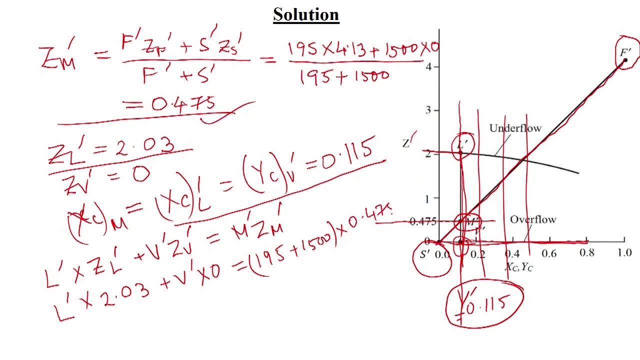 0.475, and here also V prime is equal to this: 195 plus 1500, that is we can say this: 1695 minus L prime. Okay, So we can say this: one L prime into 2.03 plus 1695 minus L prime into 0. practically it is: 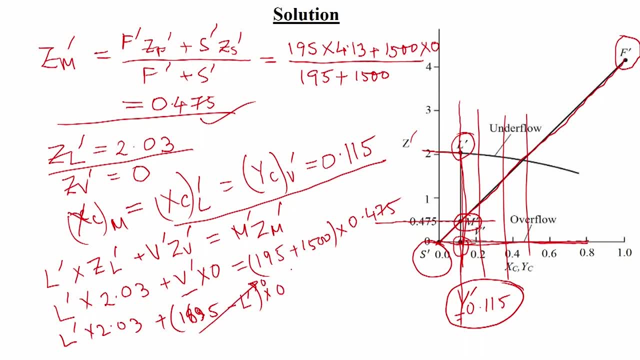 coming out as 0. So there is no need of doing this one and is equal to- we can say this- 1695 into 0.475.. So from here we are getting this L prime as this: 396.67.. Okay, Okay. 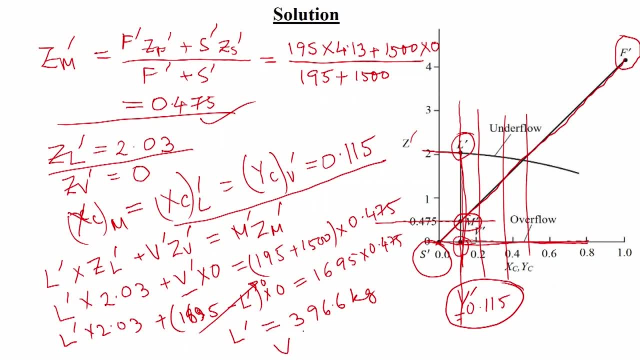 So we will be getting this. V prime is equal to 1695 minus 396.6, that is coming out at as 1298.4 kg. Okay, So we can say this one mass of this overflow, that is, we can say this one overflow that.